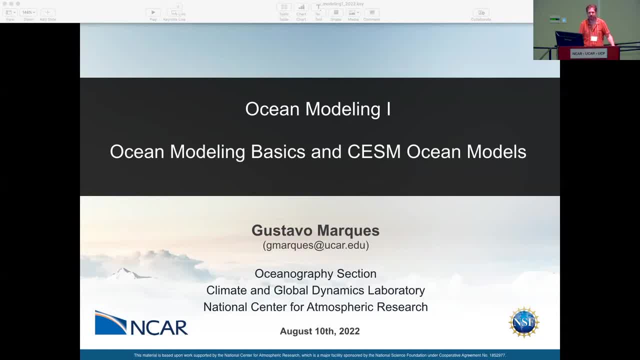 Okay, well, welcome back everyone. To change gears, we're going to be going into ocean modeling now, And so Gustavo Marquez was actually the tutorial chair last year, So he's had a lot of experience in this role. He's the liaison for the Ocean Model Working Group. That's great Yeah. 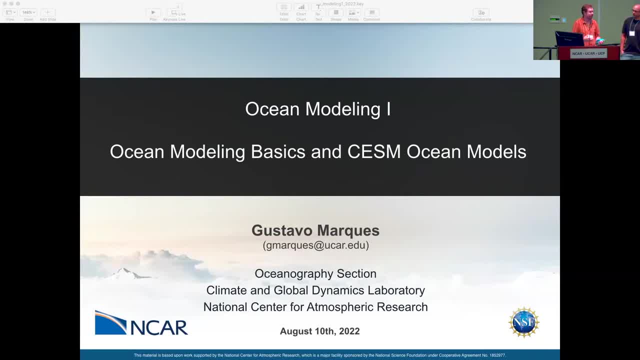 And he's been fundamental in terms of getting the transition from pop to mom going. I'll let Gustavo take over and give you some ideas about ocean modeling. Thanks, Gustavo. Good morning everybody. I'm a physical oceanography by training. 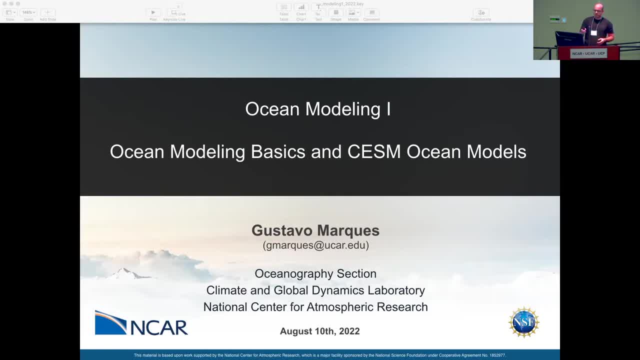 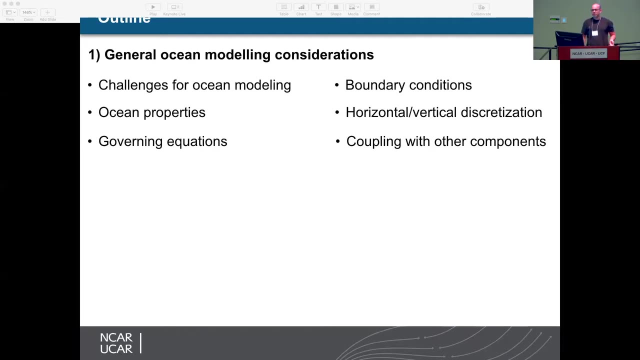 specialized in ocean modeling, project scientist in the oceanography section here at CGD. So I'll give you a perspective on the basics of ocean modeling, starting with what are the challenges? some ocean properties, the governing equations, boundary conditions, then the types of grid, horizontal and vertical. 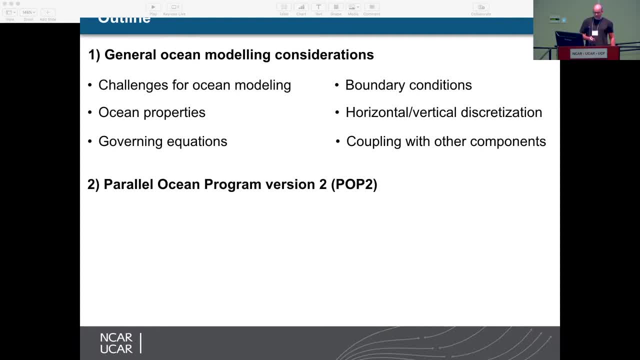 how we couple with other components. really briefly, Then I'll very quickly mention some of the characteristics of the two ocean models that we're using. So the parallel ocean model, version 2, pop, which is the ocean model that you guys are using on the practical at the moment. 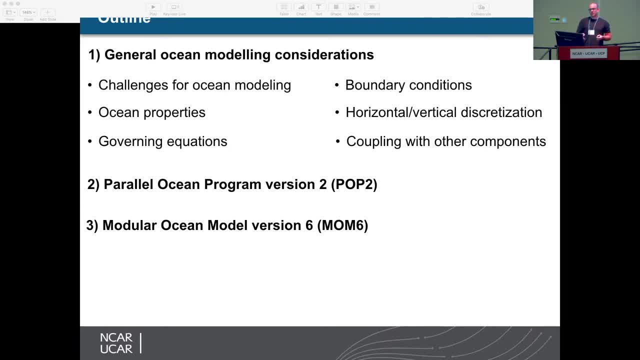 Then I'll touch upon the. I'll mention briefly about the modular ocean model version 6, or MOM 6 for short, which is the new ocean model that we are transitioning to, And I'll provide you some helpful resources. Tomorrow, Peter-Jen will focus more on the parametrization. 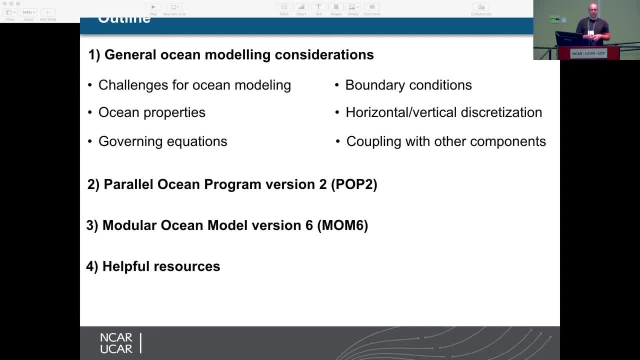 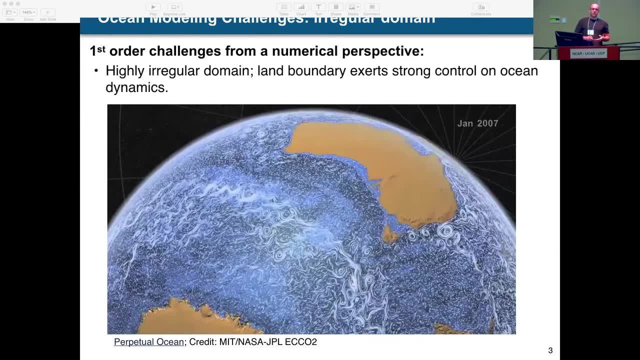 that we use in the ocean model. So today I will stay with the basic concepts and I'll give you a general overview, So let's jump right on it. The most, or I guess the other one challenge in ocean modeling is the fact that the ocean or the land boundaries are very irregular. 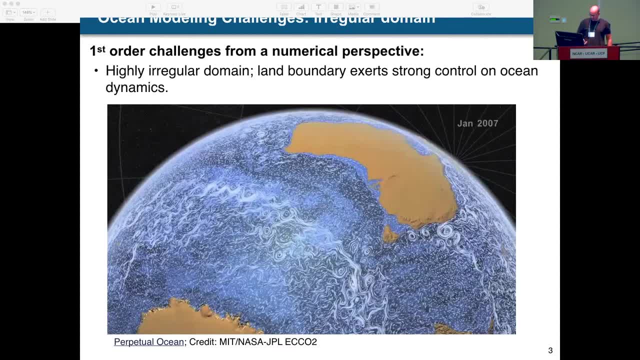 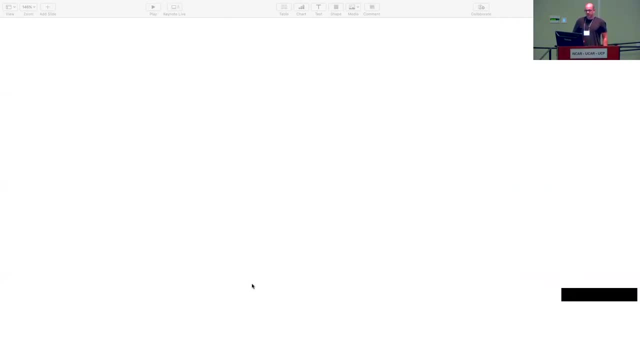 And I'll try to play this animation for you guys. How do I do that? Oops, Well, it took me to YouTube, All right. So this is the perpetual ocean from what's done with MIT, GCM, And the idea here is: these are the ocean currents, the surface currents, just to pay attention to how complex they are. 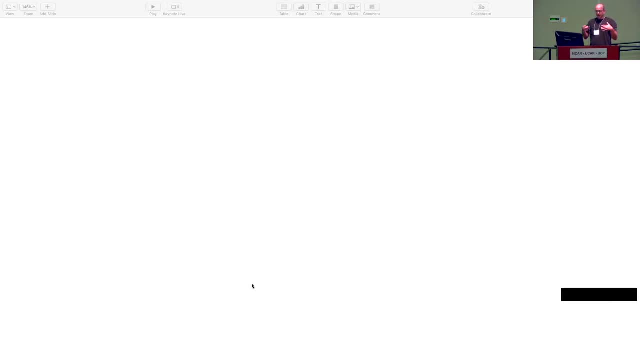 like how and how the land is playing a crucial role in kind of dictating how the currents look like, for example between Mexico and Cuba, Like they have. the current has to flow with this narrow channel and then creates this meandering and then kind of flows towards the Florida. 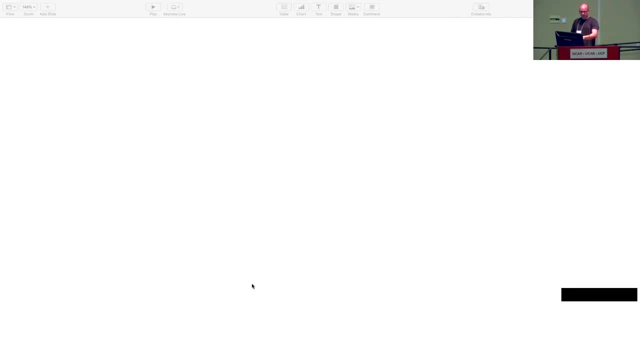 the Florida Straits and then the Gulf Stream. Now we're moving to the equatorial region in the Atlantic. a lot of eddies now to the tip of Africa. So you see the so-called Gullah's rings. look, they're formed between Madagascar and in Africa and then they kind of propagate towards the Atlantic. 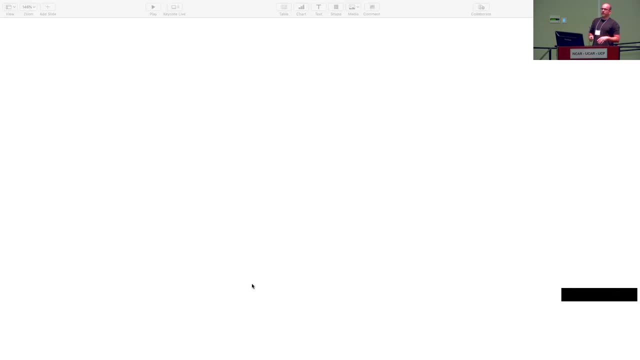 Now moving to the Indian Ocean. So I'll let you I put the link for this animation on the PDF and you guys can take a look afterwards. So just pay attention of how the regular boundaries play a key role in dictating how the ocean currents look like. 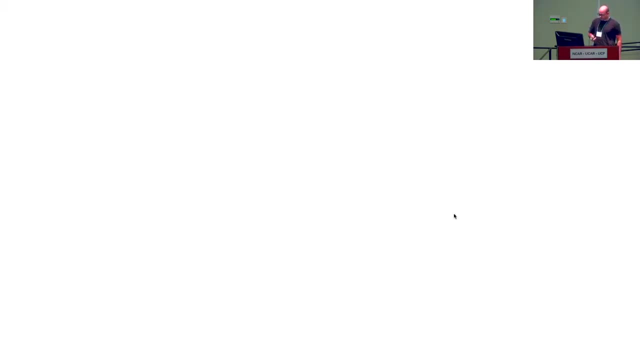 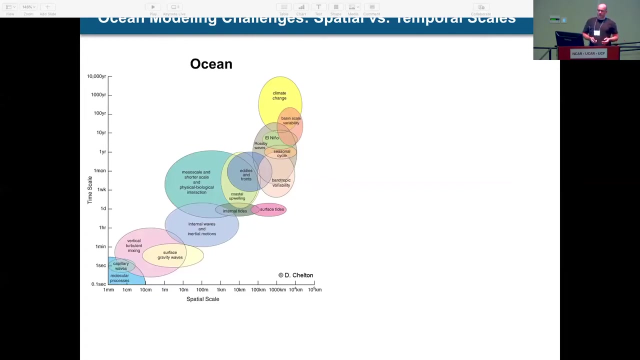 And now we can go back to the presentation. please, Thank you. This plot is showing The time scale in the y-axis versus the spatial scale on the x-axis, and you probably have seen this kind of thought before. is in logarithmic- logarithmic on both axis. 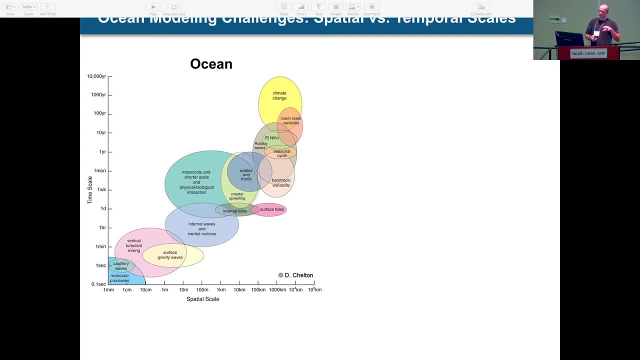 And then the balloons show kind of different processes happening. So if you go from the bottom left, those are the smallest and fastest- for example, capillary waves- to the top right, those are the long and enlarged- for example, climate change, El Nino. 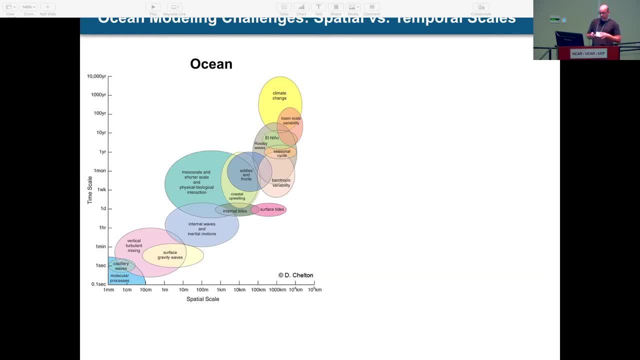 So I'm highlighting all these processes happening between the two of them. There's a lot of things going on And now, in green, these are the typical resolution, both spatially and temporal, that we resolved with the three degree ocean model. She's in the low resolution ocean model. 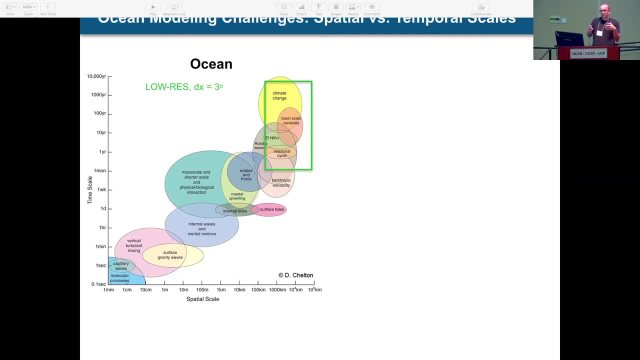 So we can capture some of the climate change like because the resolution is low, we can run for thousands of years. We can observe El Nino, some RASB waves And then now, Now in black is the workhorse when there is the grid configuration. 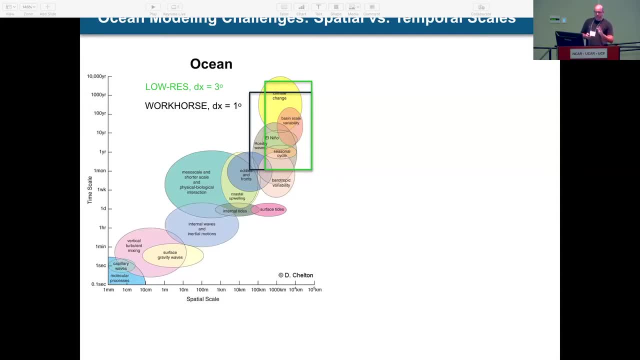 which is what you guys run on the practical example. So now we're able to go a little bit to the left and capture more spatial scales, a little bit of the eddies and fronts, but no, just very little of those processes. 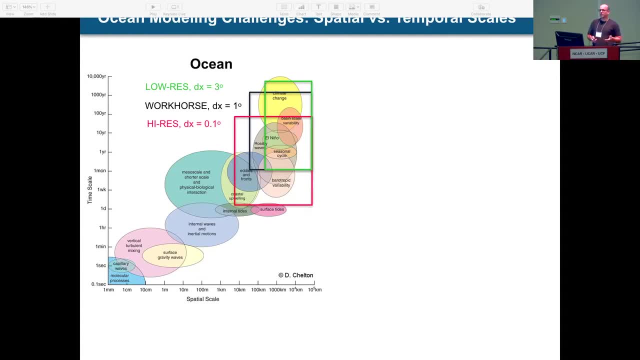 Now the high resolution grid that we have, which is a 1 10th of degree in red. now you're starting to capture most of the eddies, but a little bit of coastal up valley and just touching on, like mesoscale on shorter scales. 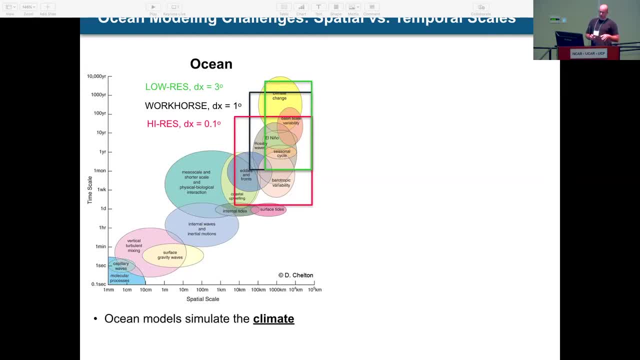 and physical, biological interaction. So the bottom line is: with ocean models we can simulate the climate. If we do the same exercise with the atmosphere, and now again with the typical workhorse configuration, one degree in the atmosphere, we are capturing most of the mesoscale with that. 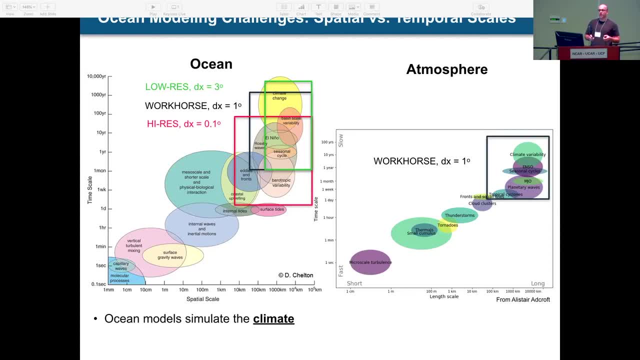 including tropical cyclone. So one degree atmosphere, we can simulate the weather. One degree ocean, we can simulate the climate. That's the big difference between these two components. And why is that? Well, I'll get on that on the next slide. 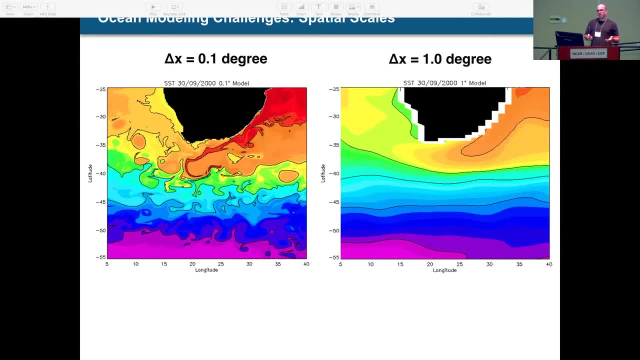 But first, the bottom line is when you use in ocean model for climate simulations, we need to come up with parameterization. So on the left is the 1 10th of degree simulation for a day, and we're looking at SST. so this is a day in 2000,. 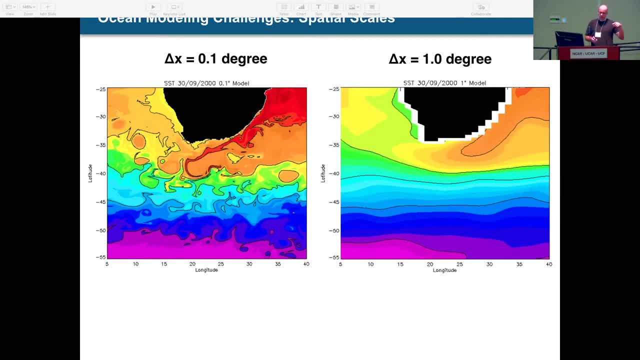 and we're looking at the tip of Africa. so those are ghoulish rings that we saw in the animation And we can see the ghoulish rings like playing it's reflection on the SSG. So you see these blobs of SSG moving to the west. 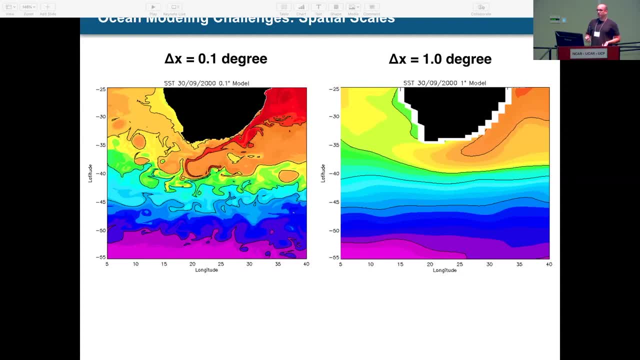 And if you look on the right, this is the same plot for a one degree on the same day And we don't see those eddies. So we need to represent on the one degree, we need to represent the fact of these eddies. 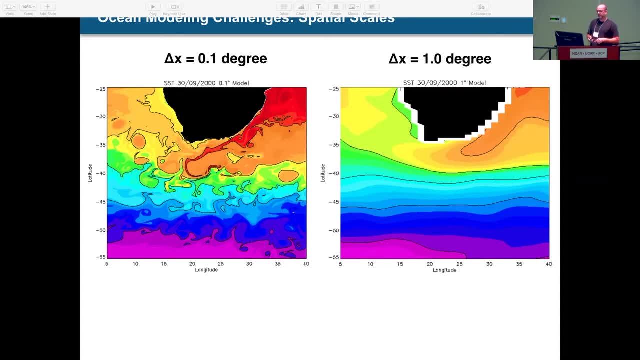 and how we do that. you will learn more about this specific type of parametrization tomorrow with Peter J. So the mixing associated with these eddies needs to be represented in the low resolution model and must be parametrized. So, going back to the difference, 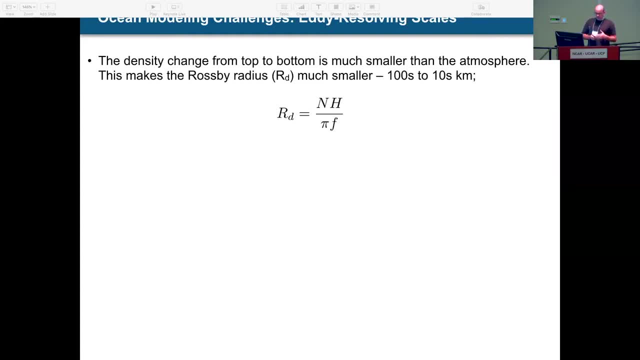 between the ocean and the atmosphere. the changes in density from the top of the atmosphere to the bottom of the atmosphere are much larger than in the ocean, And that affects the so-called Rosby ranges of deformation, which is given here. So N is the Broom-Weieraro frequency. 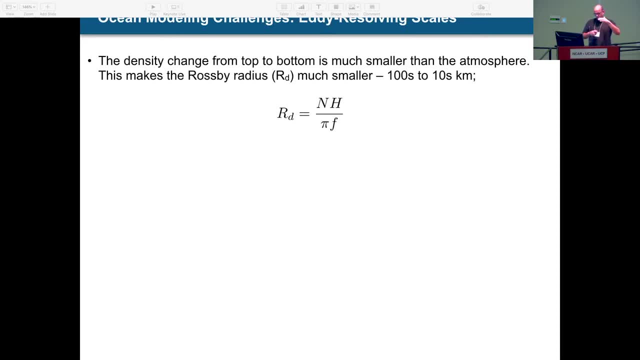 H is the vertical dimension of the domain and then, on divided by PI, F is the Coriolis parameter. So in the ocean, the first radius of deformations on the order of hundreds to tens of kilometers, while in the atmosphere is another magnitude larger. 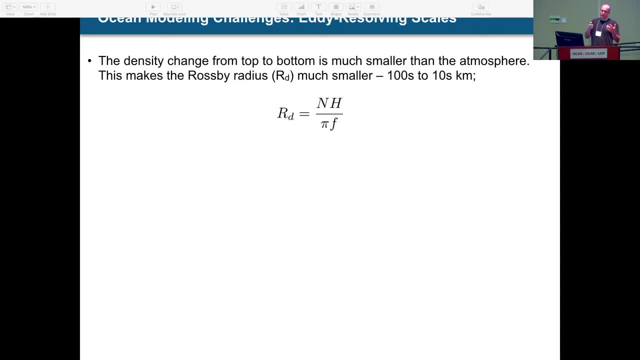 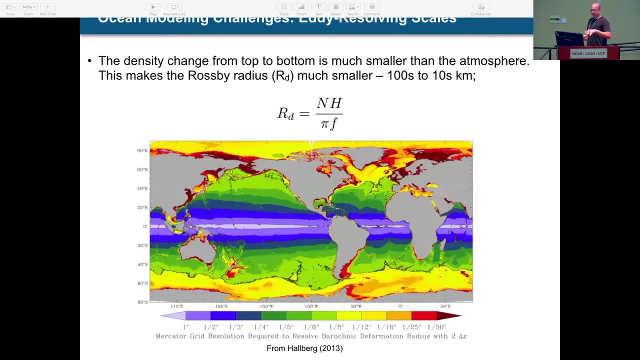 therefore, like it's, you need less. you need less grid spacing to represent, or you need a with a coarser resolution grid space. you can represent better the mesoscale process in the atmosphere compared to the ocean And, to give you an idea, this plot is from Halberg 2013.. 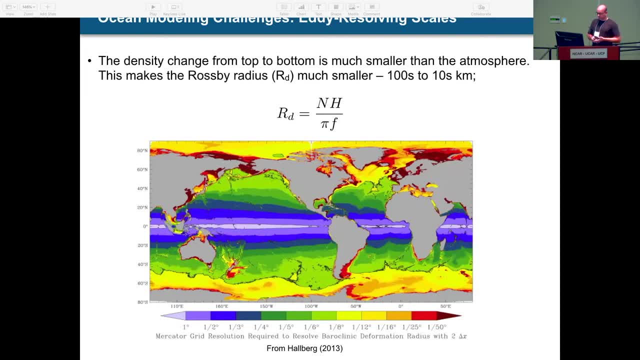 It shows the is the ratio between the bioclinic rates of deformation divided by the grid spacing. So you can just to give you an idea of like how much resolution in the horizontal is needed to start resolving the mesoscale eddies. 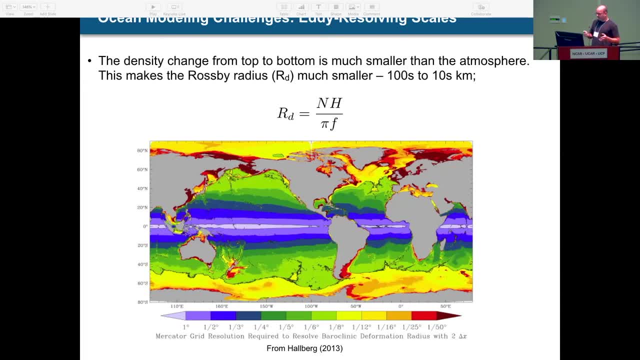 So in the equator is on the order of between one and half a degree, like that, And it's really showing here it's. the radius is like two Delta X, So two times the grid spacing And in reality we need like at least six times. 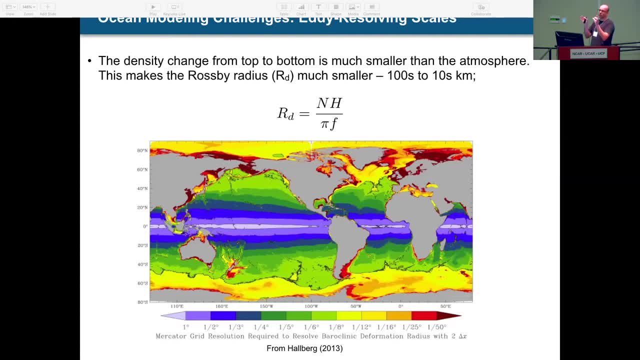 So you need, within one radius of deformation, six grid points in order to resolve well the mesoscale phenomenon. So you know it's even worse than what's shown here, but the bottom line is in the equator You need order of like half of the grid. 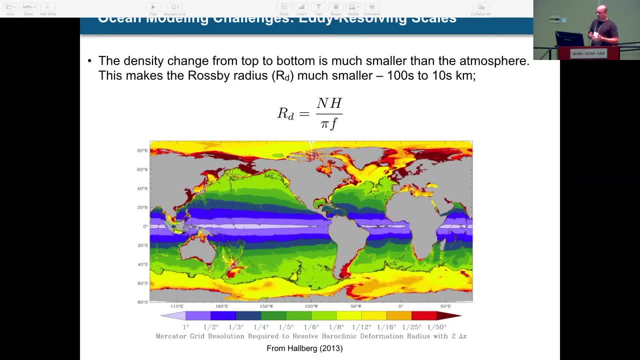 to start resolving the first bioclinic of deformation, while at high latitudes, like it's kind of off the scale, here it's like less than one 50th of a degree, A one 10th of a degree, you can resolve the mesoscale mostly everywhere. 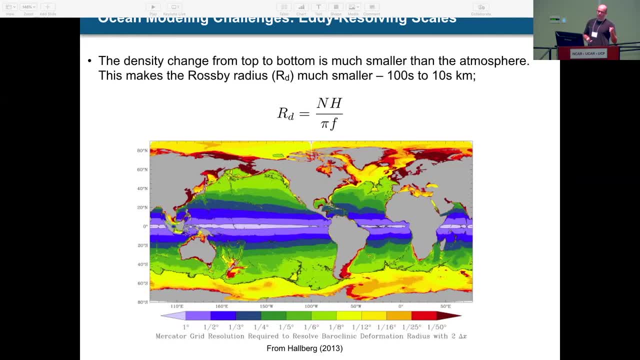 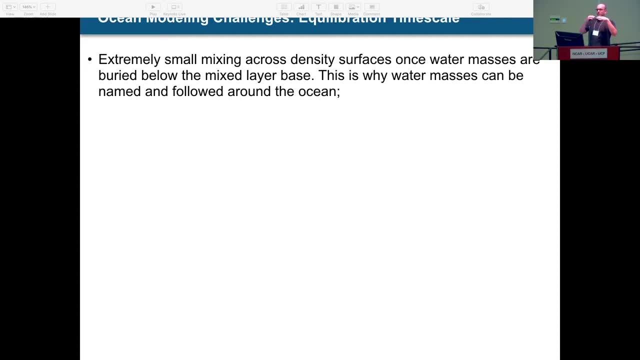 but still not at all locations, especially high latitudes and shallow. Another challenge in ocean modeling is that was the water masses are four and they sink below the surface. There's very little mixing that happens between them and that's why we can name the water masses. you've probably heard 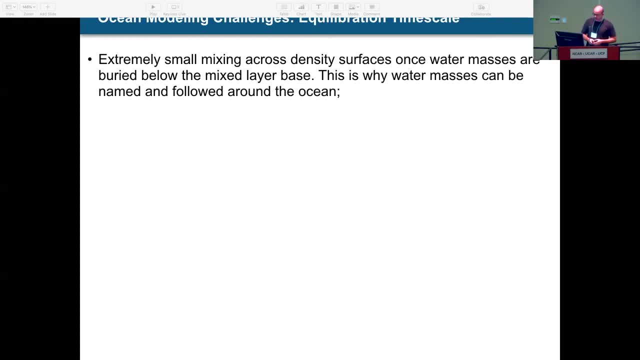 it when the tolerable water- North Brian Grande, North Atlantic, deep water And these are- is actually a challenge for in terms of representing ocean with computers, because any numerical spurious mixing will affect your solution a lot. So, like you know, you need to make the solution small. 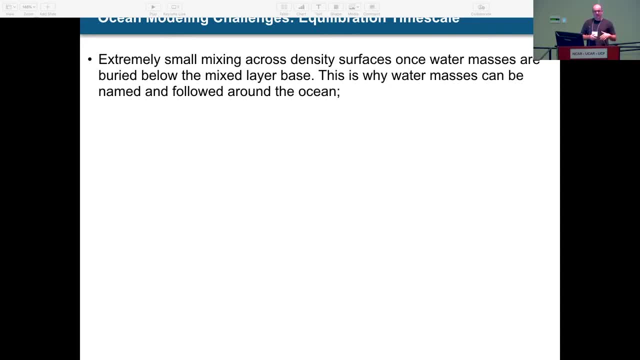 need to. once the water masses are formed and they sink again, very little mixing that happens and any spurious mixing because of your numerics will affect your solution, especially in climate simulations. Another challenge is because the deep ocean that there's like little mixing. 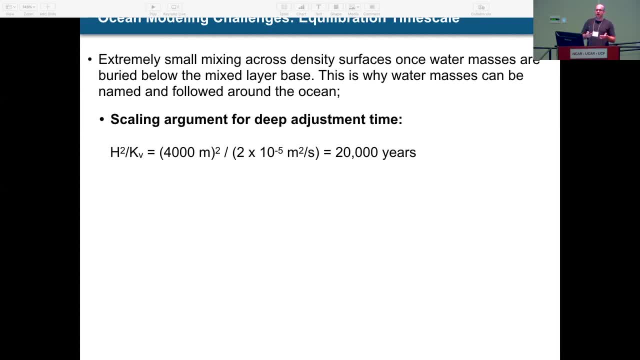 you can use a simple scaling argument to estimate how long you will take for the deep ocean to equilibrate. So if you take like typical vertical scale of the ocean, like the typical depth of the ocean on average is like 4,000 meter. 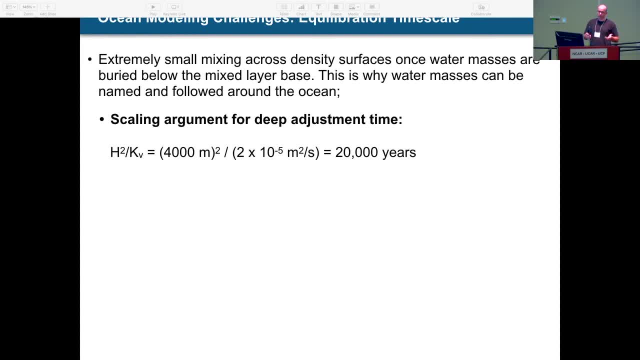 you square that and divide it by the vertical diffusivity- like no typical vertical diffusivity used- you get a 20,000 years. So that's approximately how long it will take for the deep ocean to equilibrate. That's a lot of time. 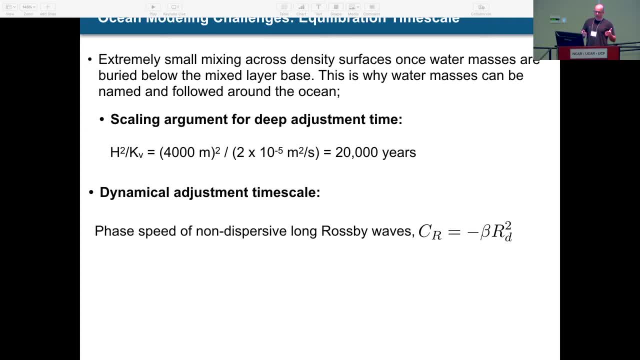 In contrast, if you just look at the dynamical adjustment time. so how long it takes for, for example, a non-dispersive long-ross buoy to cross the ocean basin- And here I'm using this dispersion relation for this kind of waves- given by C sub R? 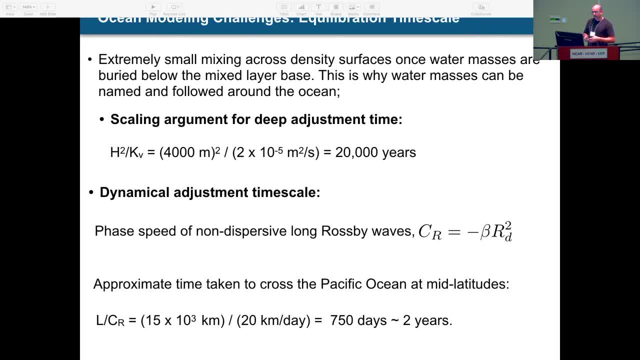 And if you take the Pacific ocean as an example, it will take approximately two years for this wave to propagate, which, compared to 20,000 years, is very fast, But compared to the atmosphere, like how long it takes from front to propagate. 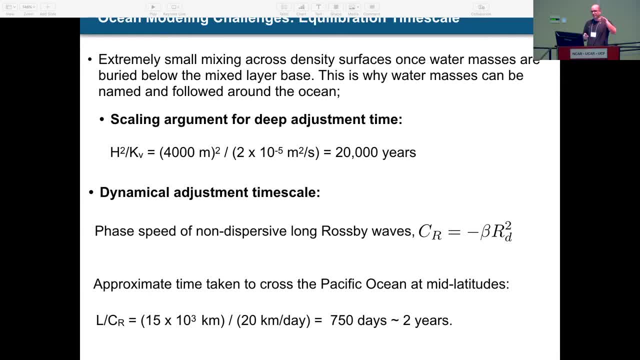 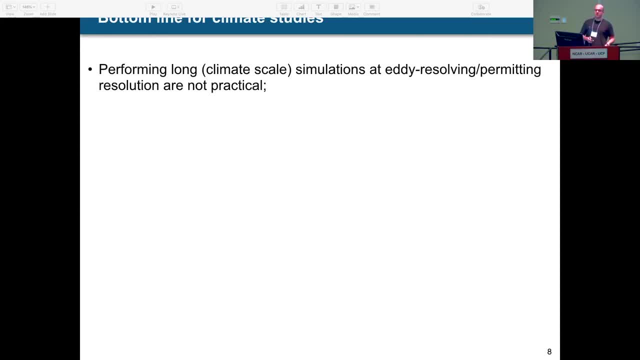 two years is very long. If you do an analogy with the same kind of phenomenon, it would be the same kind of phenomenon in the atmosphere, which is much faster. The bottom line is that performing climate simulations along climate simulations with at resolving or permitting models is unpractical. 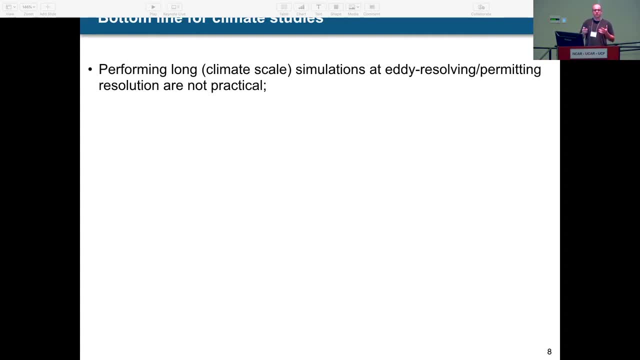 because we need a lot of resolution. Therefore, we use, like we tend to use, a resolution that requires podometrizations, especially for these long simulations. The spurious mixing in the ocean is a big deal and significantly degraded the solution. 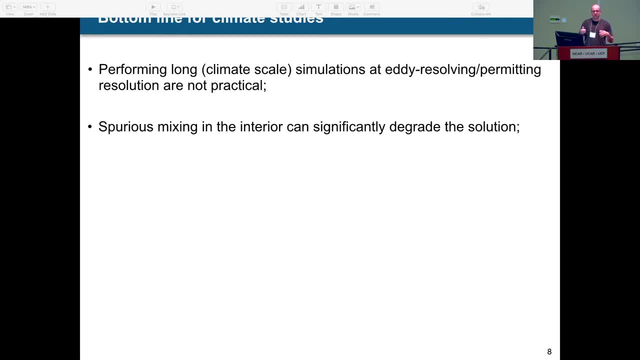 So when we design ocean models for climate simulations, we have to be very careful with that And we must leave with the ocean not being at equilibrium. That is very rarely you see a simulation that was run for thousands of years. It's mostly done for paleo. 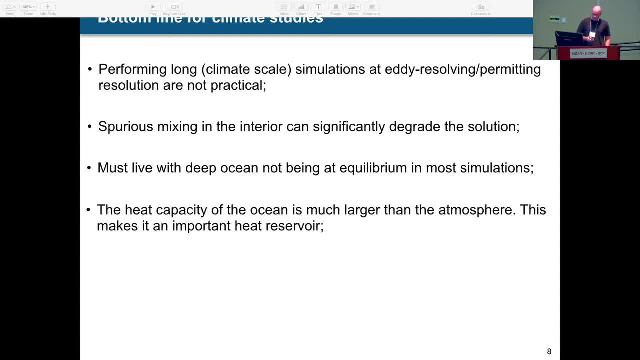 And those things should be very coarse resolution. And another thing that I didn't mention is that the heat capacity in the ocean is much larger than the atmosphere. That's a big deal because the ocean is an important reservoir for heat. So the ocean has been taking all the excessive heat. 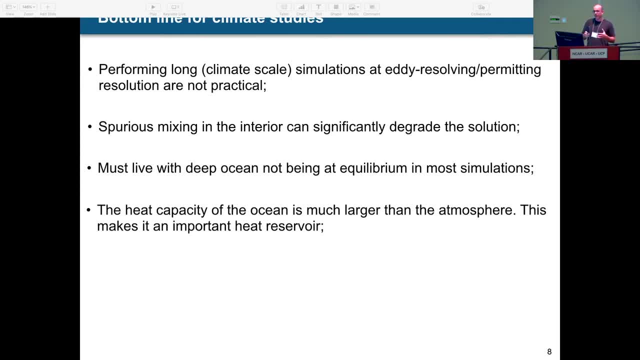 that is being given by climate change and how will that affect us? No, we're still trying to understand that, But all that excessive heat is being accumulated in the ocean And because of this, the ocean has the memory for the climate system and has a lot of implications. 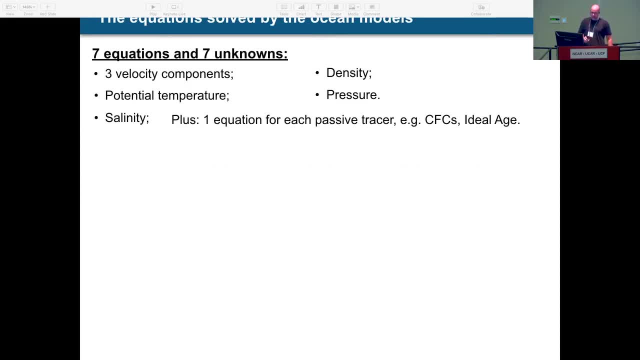 for things like climate change, Like decadal prediction and so on. Okay, so now moving to the equations governing the ocean. I'll try to simplify as much as possible. I'm kind of giving you a general sense here. Keep in mind that there's a lot of details. 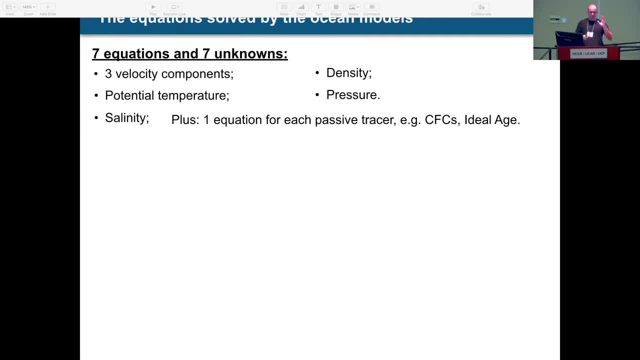 that are not included here, but I'm happy to talk afterwards with those of you interested in like going to the weeds. So we have seven equations and seven unknowns. So we have three equations for velocity, u, v, w, One equation for potential temperature. 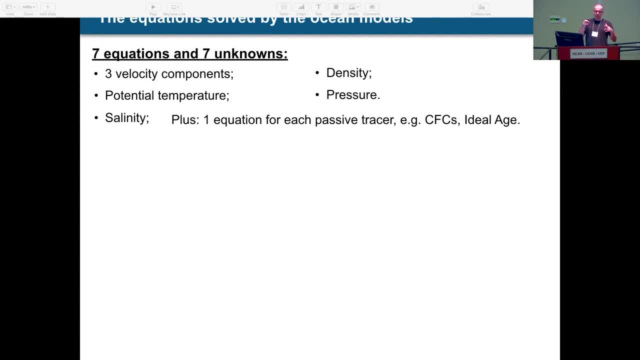 One equation for salinity, then density, which combines both potential temperature and salinity, and then pressure. So with seven equations, seven unknowns, we can solve this system. Plus if you have all the traces, for example CFCs, ideal age, 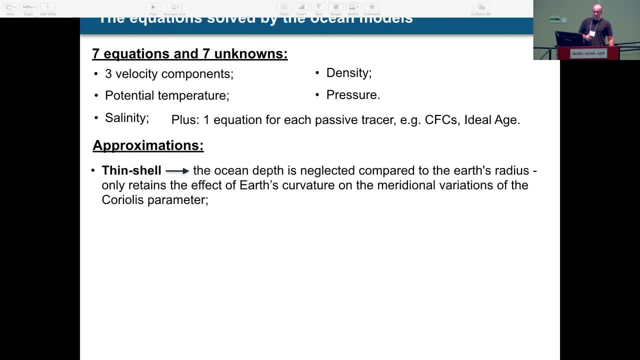 then you need a separate equation for each of those. The approximations that are made when we designed the ocean models are: the first one is a thin shell. Basically, the depth of the ocean can be neglected when compared to the radius of the earth, And that leads to like simplifications. 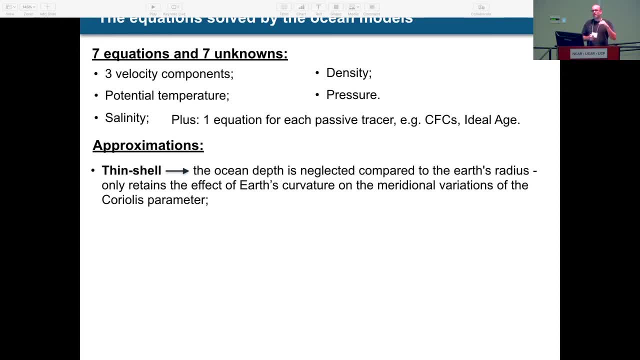 in the Mariana variation of, sorry, in the zonal variation of the Coriolis pattern. So we only consider the curvature effect in Coriolis on the Mariana direction, not in the zonal, The Boussinesq approximation, which is a big deal. 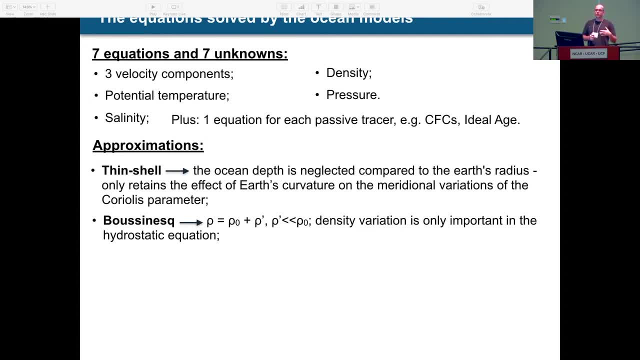 basically, the changes in the density of the ocean are very small when compared to the mean density, And that's what is given here. So, rho, you can approximate rho as rho-nau plus rho-prime, where rho-prime is much smaller than rho-nau. 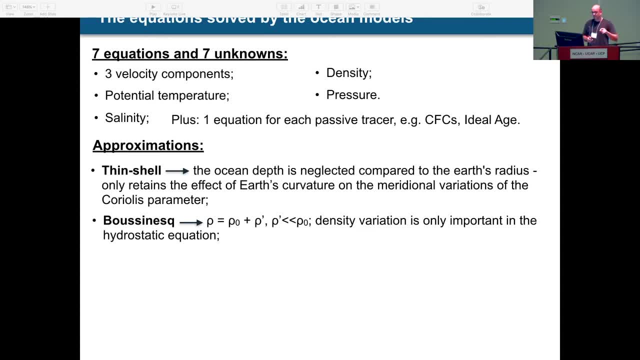 Therefore, like everywhere in the equations, but in the hydrostatic approximation, we can replace rho by rho-nau Continuity equation. so basically incompressible flow. So what flows into a control volume, what flows in must flow out. So it's the idea of constant volume in the ocean. 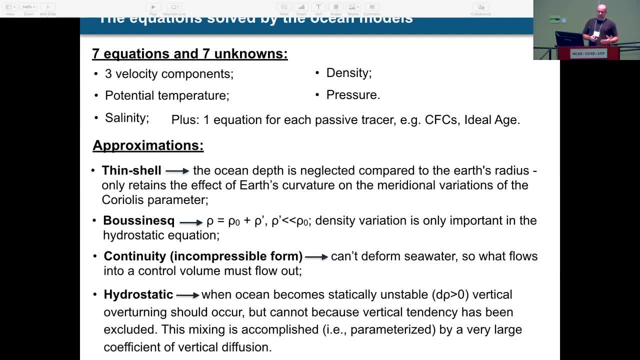 And then finally the hydrostatic approximation, which basically all the vertical accelerations that are smaller than gravity are neglected, And for climate ocean model using climate simulations. this is a pretty good approximation If you go more into like coastal ocean modeling. 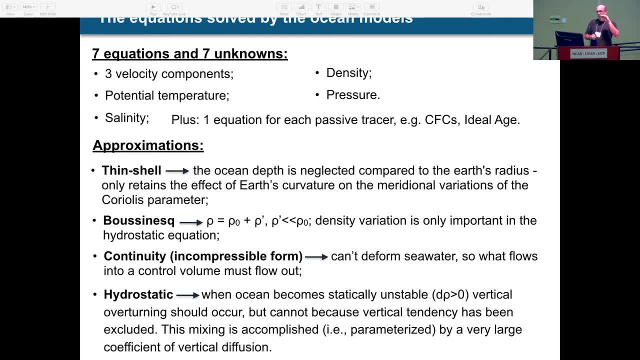 then this starts to break, because then your horizontal and vertical scales become more comparable And things like Kelvin-Helmholtz instability- you can start to it- becomes more important and you can start to represent them, But like in a global climate model. 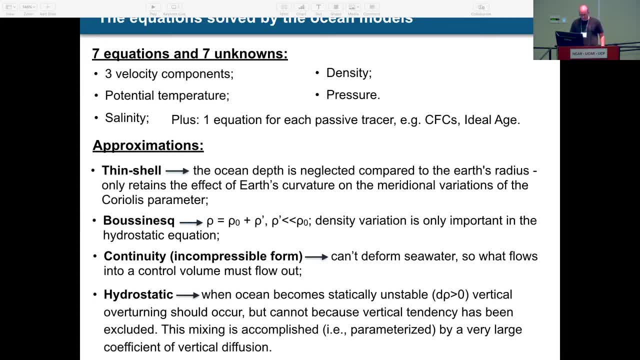 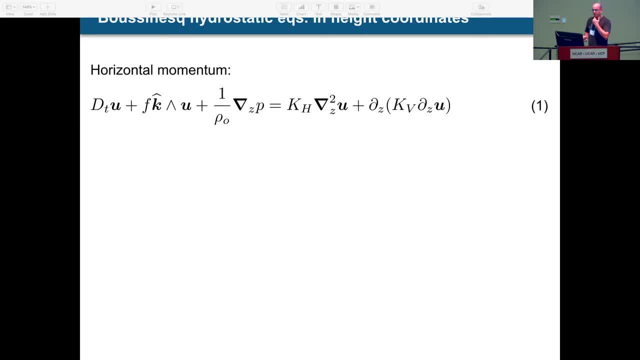 you cannot represent things like that, like these type of instabilities. That's why the hydrostatic approximation is a good one for these cases. So, jumping into the equations, this is the equation for horizontal momentum in vector form. This is the vertical momentous or hydrostatic approximation. 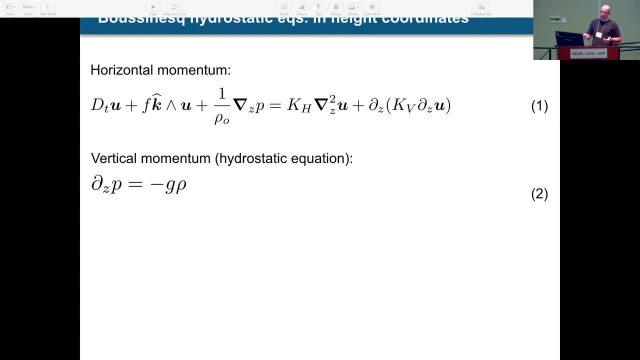 So basically, partial z equals minus rho g, Mass conservation, which is now 3a. So in this equation we have a two form of mass conservation, but because we make the hydrostatic approximation, that simplifies into the continuo equation. 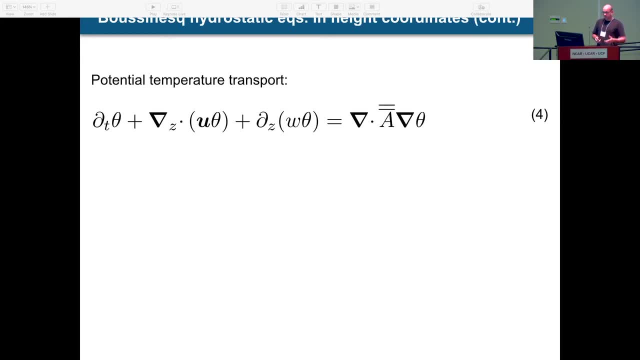 which is given by 3b, The transport of temperature. and, by the way, I'm neglecting the sources and sinks on the right hand side here. So, like the same for the momentum equations you have. like, the forcing at the surface is not included here. 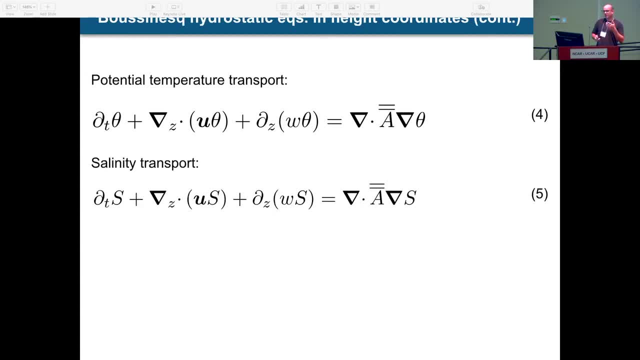 but I will talk about that a little bit. So this is for temperature, Similarly for salinities, the same equation. Finally, equation of state, which is a nonlinear equation where we combine salinity, potential temperature and pressure to give you density. 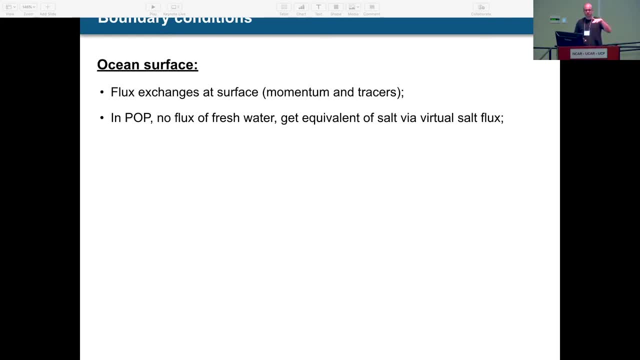 What are the boundary conditions? So, starting from the ocean surface, there are flux exchanges at the surface, for example momentum, the wind blowing on top of the ocean, also heat and fresh water. So heat goes into the temperature equation, fresh water goes into the salinity equation and mass. 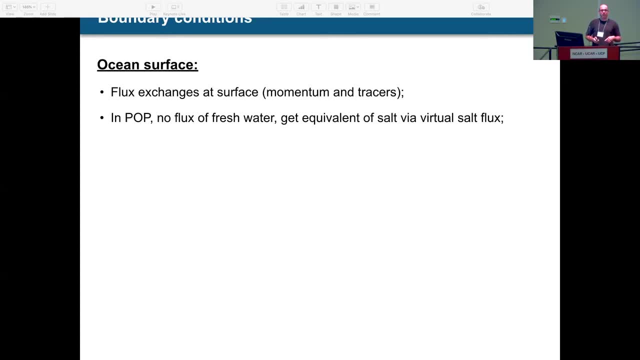 Important to note that in POP, in the POP model, the one that you guys are using, there is no fresh water flux And instead we do something called virtual salt flux. So if rains on top of the ocean, instead of throwing fresh water into the ocean, 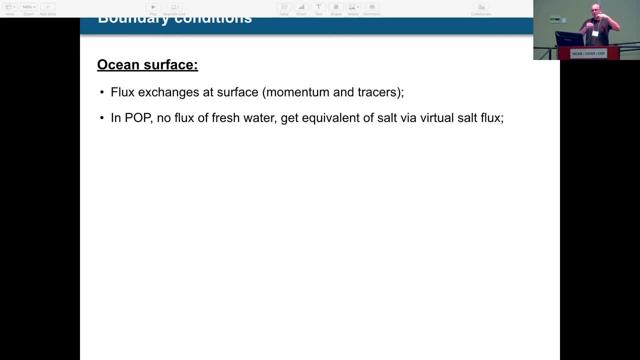 we just. we take or put salt, depending on if you're throwing water. you're diluting the ocean. So we will remove salt to kind of mimic what was happening if you were diluting the ocean. It's only in POP, In MOM. it uses the so-called natural boundary condition. 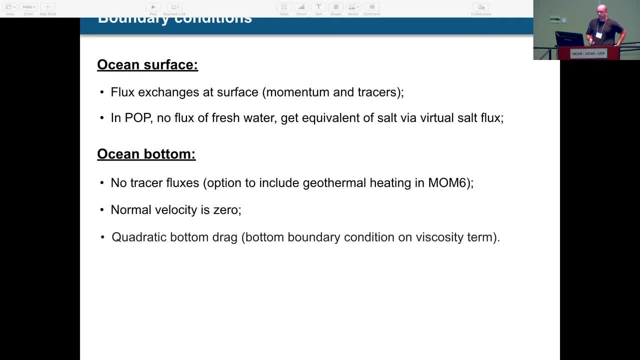 where you can actually put water, add water In the ocean bottom. we have no traces through the no traces flux through the bottom. There is an option in MOM to represent geothermal heating, but we're not exercising that at the moment. 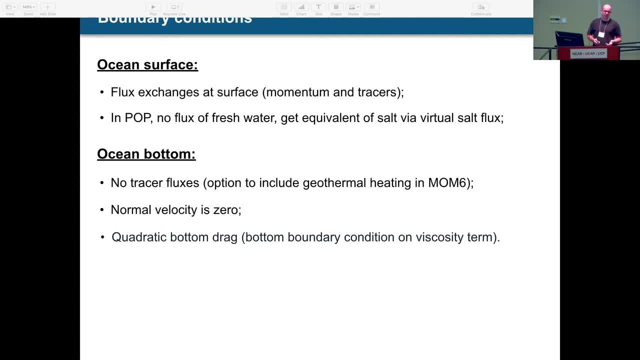 And the normal velocity is such a zero And then we have a quadratic bottom stress. Then the lateral boundaries are no tracer, no fluxes through Through the boundaries And the flow normal to the solid boundary section is zero And there's also no slip boundary conditions at the sides. 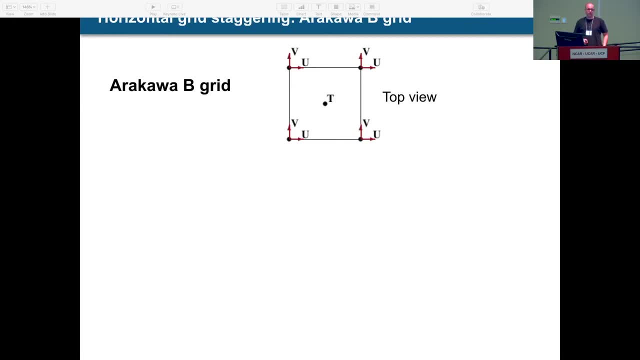 Now, moving to the type of horizontal grid staggering used. I'm gonna present you two, because the two models that we are working on have different staggering, starting with the so-called Arakawa B-grid, which is shown here, So in at the center of the cell in the letter T. 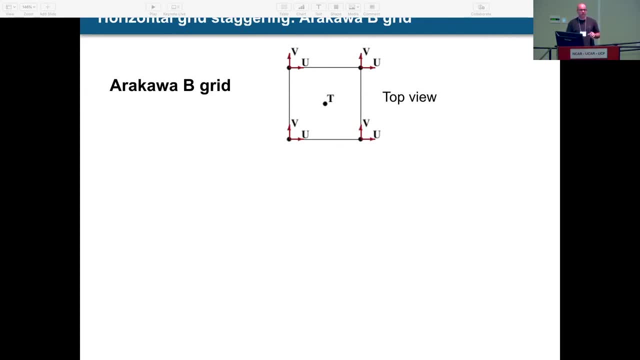 those are tracer points And then the corners U and V. that's where we represent the velocity points. So no, they're not on the same point, They're kind of co-located. This is a top view, And the advantage of this grid is that it naturally fits. 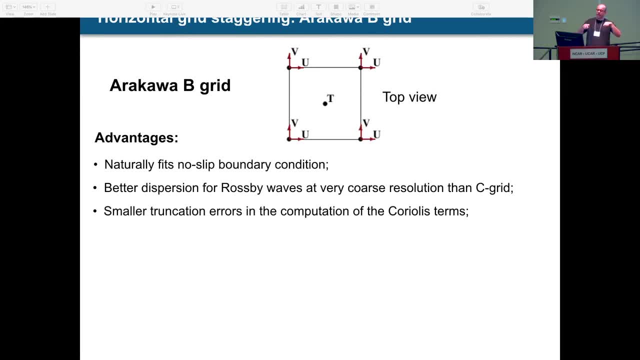 the no slip boundary conditions. So U and V on the same point is easy to say: oh, this is land, So it's supposed to be zero. So imposing the no slip boundary condition is easier on this grid. It has a better dispersion of the Rossby waves. 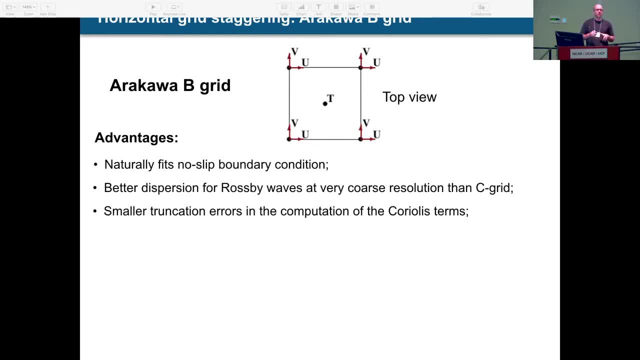 at coarse resolution. So again those paleo type simulations that have very coarse resolution, three degrees or so. the B-grid has advantage over other grades And also has these small altercation errors in the computation of the Coriolis term. So that's the minus VU plus VF, minus FU plus FV. 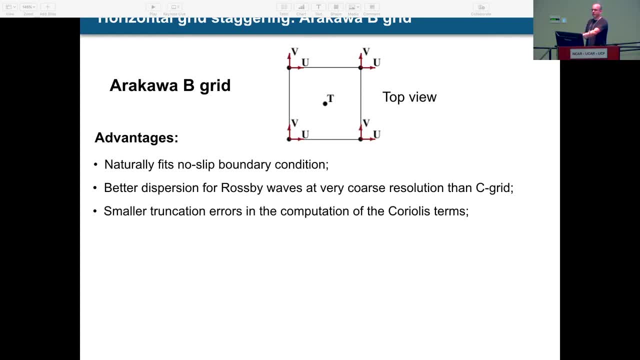 in the momentum equations Because U and V are on the same point in this grid. we don't need to do interpolation of the, the components to do to calculate the Coriolis term, which is helpful and leads to small altercation errors. 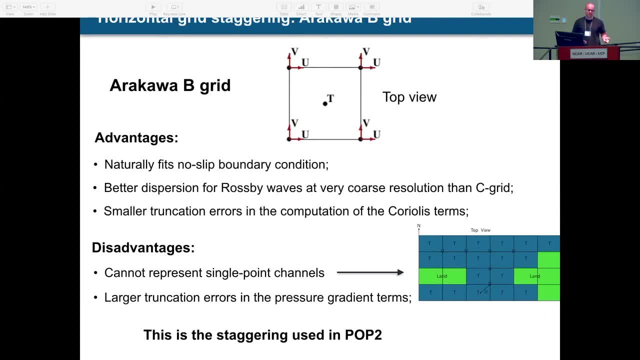 The disadvantage is that we cannot represent, first of all, we cannot represent- single point channels. So, as shown in this schematic on the right, the green squares are land, the blue are ocean- In order to have a channel that the water flows through, 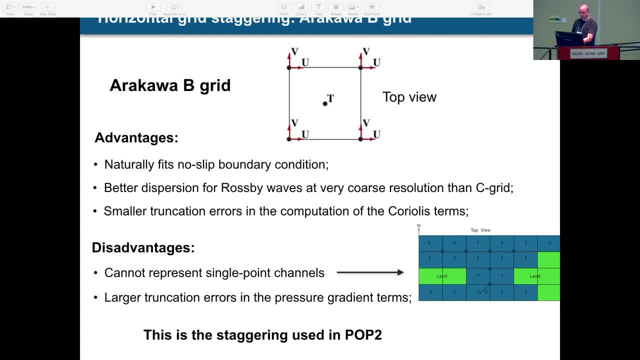 you need to have at least two grid points, So two as shown by the capital T here, otherwise the velocity points will always be on land and you will not be able to to flow through through that, that that channel. 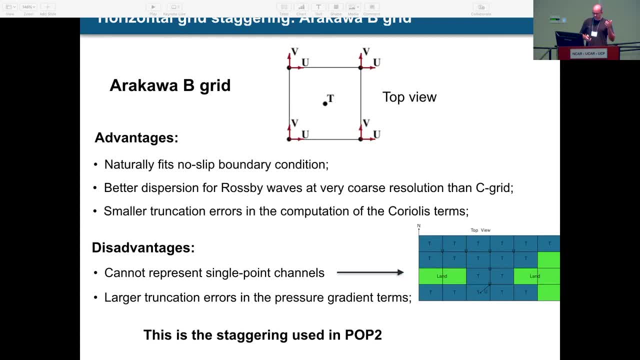 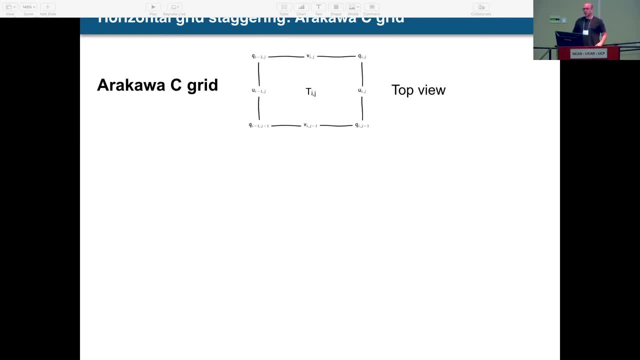 And it also has large altercations in the pressure gradient terms. So, as I mentioned before, this is the grid that we use in the pop model that you guys are running right now. The other grid is the so-called Arakawa C-grid. 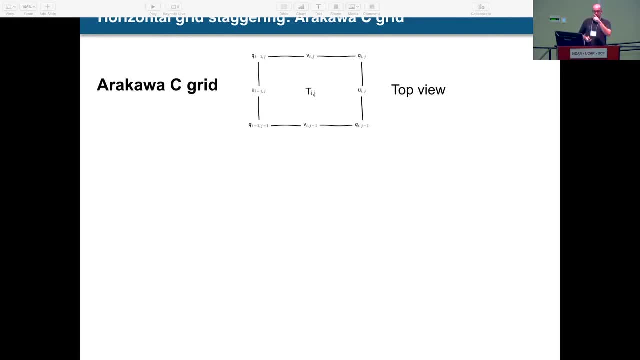 And so again, the tracer points are on the center, but now U and V are co-located, So U is on the side of of the tracer points and V is on top and bottom. Again, this top view highlights that. 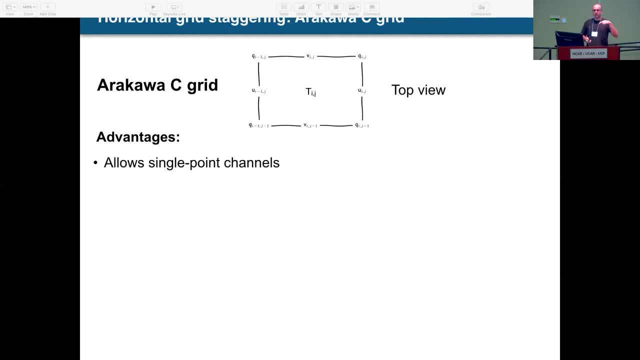 And what is the? the main advantage of this is that you can now simulate the flow through a channel using a single grid cell, Because even though U will be masked- like, let's say, you have land on both your left and right side- the U points will be masked. 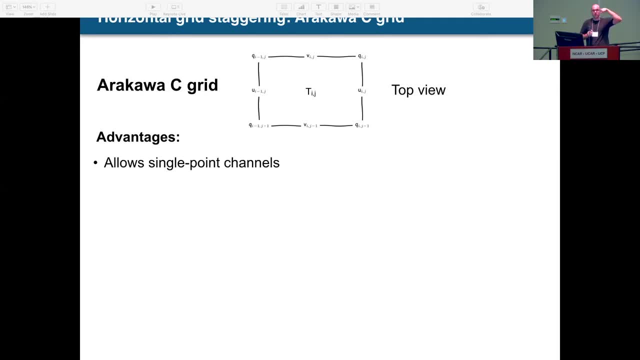 You will now have a zone of flux, but the V points will be ocean and you'll be able to flow through through the channel, And then the disadvantage is kind of the opposite of the advantage of the other one. So there is a, the Coriolis terms. 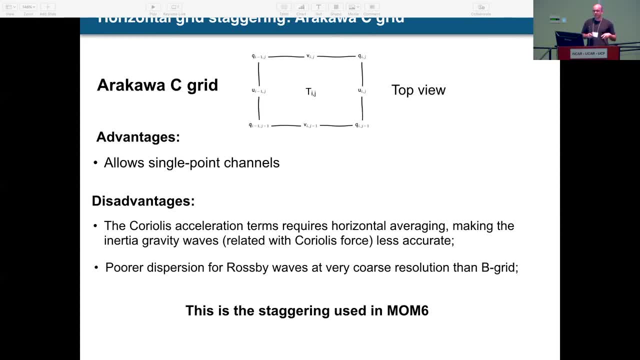 now you need to do interpolation because U and V are on different locations And then you have a, didn't you have a? no, it's less accurate than accurate than in the B-grid, And it also has not not as good dispersion relations. 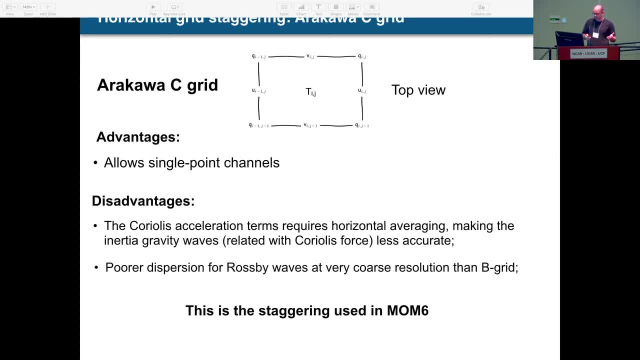 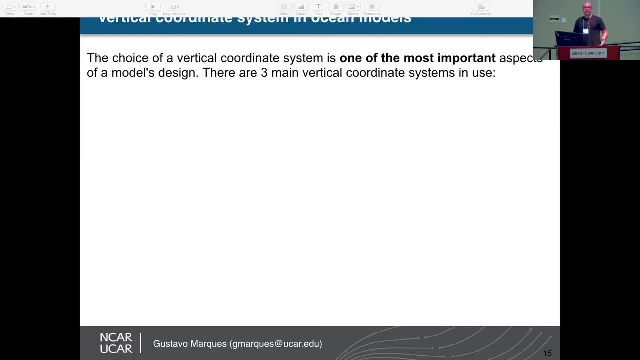 for the Rossby waves at coarse resolution, So like three degrees or so, And this is the grid used in the MOM6 model: The choice of vertical coordinate systems in the OSHA model. So this is a very important topic of research And when you're designing the OSHA model. 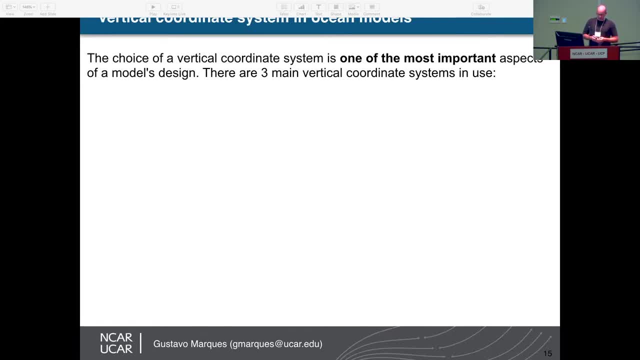 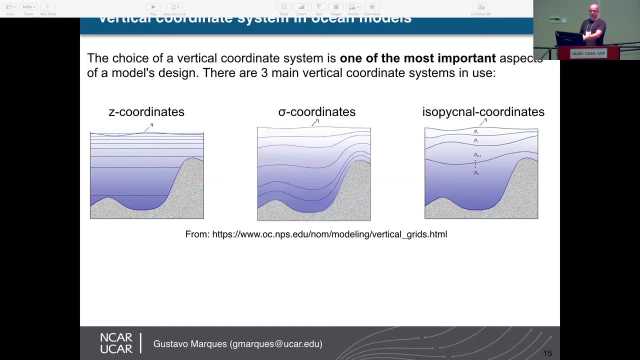 your choice of vertical coordinate system makes a huge difference And I'm gonna list you like three different coordinate systems that are used. Like most of the models use the Z coordinates, So the first one on the left. The main advantage of this coordinate is: 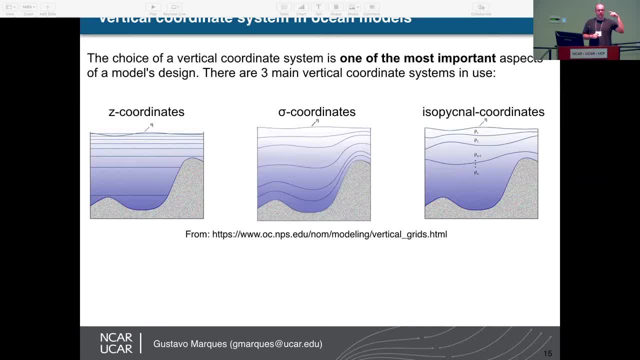 this is basically. your coordinate is a function of that, And you can specify the resolution on the water column where you would like And that resolution will be fixed throughout the simulation. The advantage of these is, like we locations, where you have a lot of mixing. 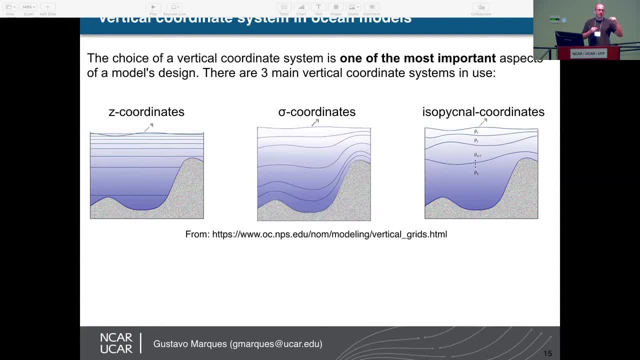 so near the surface. you can put a lot of points there and represent the processes happening there well. It's advantage, however, is that as you go your topography towards the bottom of the ocean, then you start having a lot of the grid space. 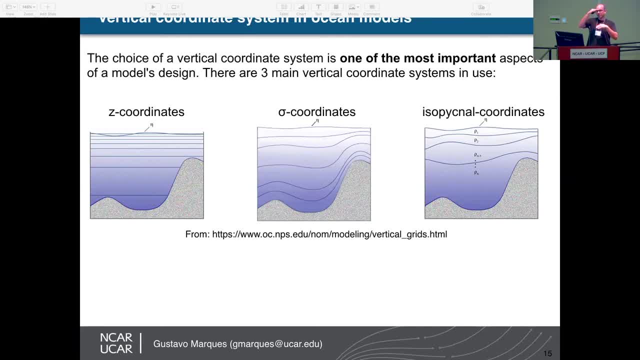 in between two interfaces. the distance between two interfaces becomes large, And then you don't represent the dynamics close to the bottom very well. You can argue that if you have a lot of grid points, then you can make a good resolution near the bottom as well. 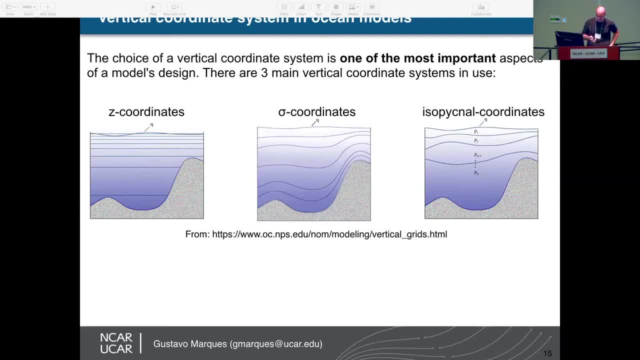 but then your model will become very computationally expensive. Another advantage is much easier to work with the equations in the Z coordinate system. Sorry, the second one on the middle is the so-called sigma or terrain falling coordinate. It's mostly used in the regional modeling community. 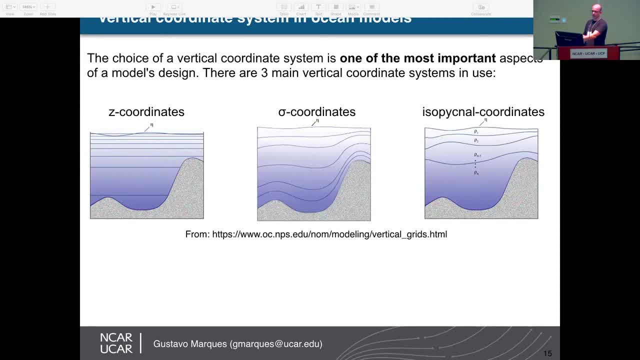 So in this case the coordinate is following the topography. Notice how the lines are kind of following the topography. Again, it's nice now because you can put the resolution you want. So you can increase resolution at the bottom, near the surface, but the main downside. 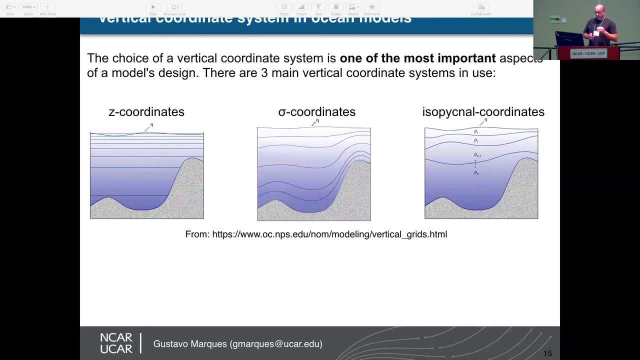 is that you can put the resolution you want. but the main downside is that you think you have a lot of pressure gradient errors near steep topography with this type of coordinate system And again, if for climate simulations, if you have any spurious mixing. 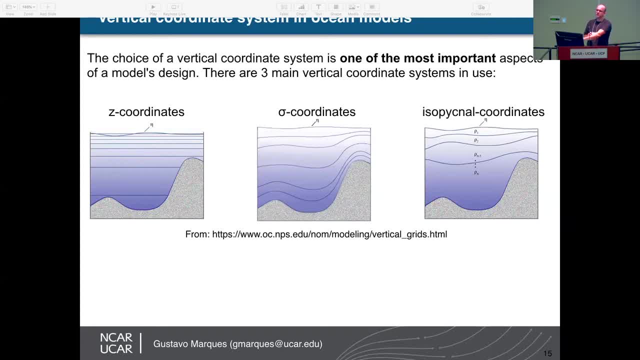 you degrade the solution a lot. So, therefore, like you rarely see ocean models used for climate simulations written in the so-called sigma coordinate. And finally, on the far right, these are the isopic coordinates. So, basically now, your coordinate is a function of: 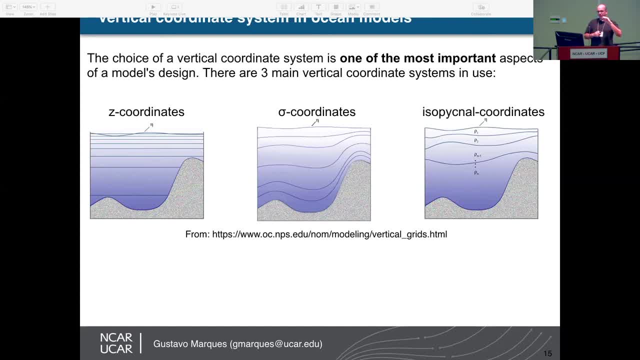 you being your coordinate in terms of density classes. So, for example, the first layer can be a potential density and we tend to use the potential density reference to 2000 deciBars, but you could use to another pressure level And then your layers have constant potential density. 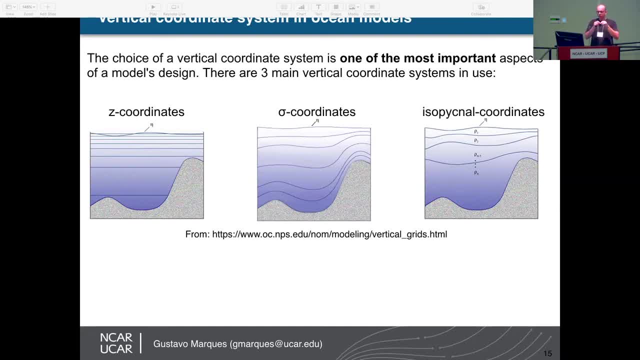 and you can then spread how you want to define it, how you want to be the density To create your coordinate. The main advantage is again now: once the water masses form and they sink, they tend to mix along density surfaces And this type of model will let you very small, spurious mixing. 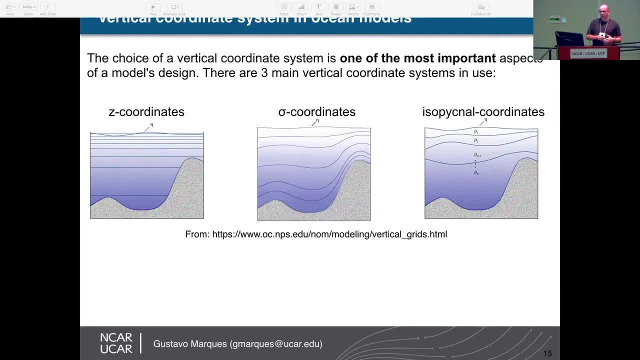 because it's a natural coordinate of the model. However, near the surface, where you have a lot of mixing, then this is an advantage of this model because it becomes. you need to combine that with a mixed layer model in order to represent, for example, 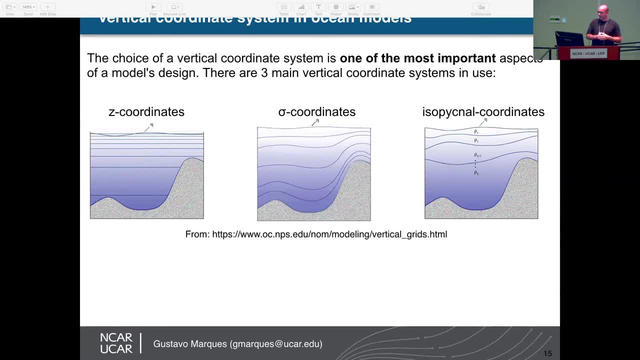 the mixing with the surface or from heating cooling. So, in reality, like we would combine all of the best of all of these and create a grid, And that's what has led to the development of the so-called hybrid coordinate systems, which is we have this capability in the new model MOM6.. 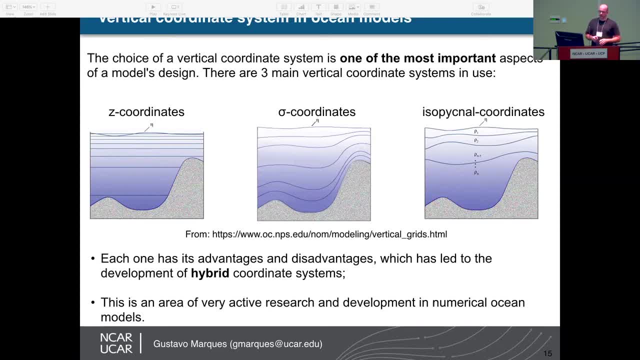 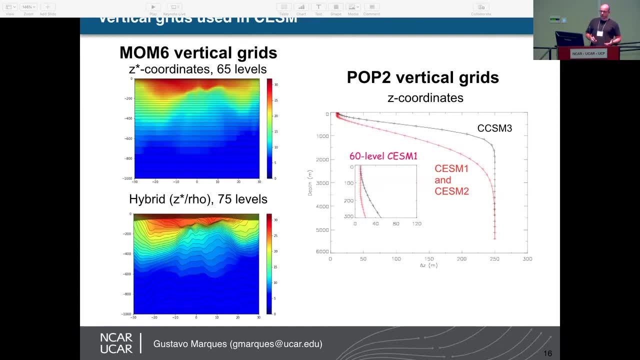 And again I want to emphasize that the coordinate system in the ocean model is an area of very active research and development. Now, focusing on the grids that we are using, So on the left are the MOM6 vertical grids, So the top is a Z coordinate. 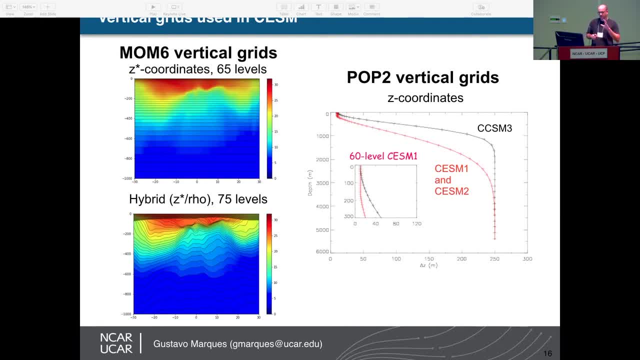 So I put Z star. So Z star is a class of the Z coordinate. Is this kind of the same idea? We have 65 levels. This is just a section of temperature and the lines represent the vertical grid. Then the bottom is a hybrid coordinate. 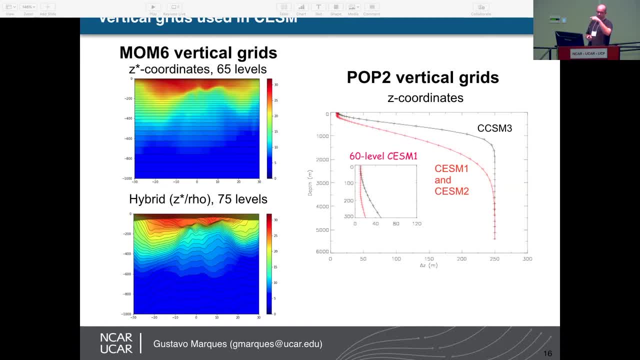 Is a Z star near the surface. So you can see, near the surface has a lot of resolution and then below a certain depth or a certain density class, we start to transition to a density coordinate And on the right, the POP vertical grids, which are all Z Star. 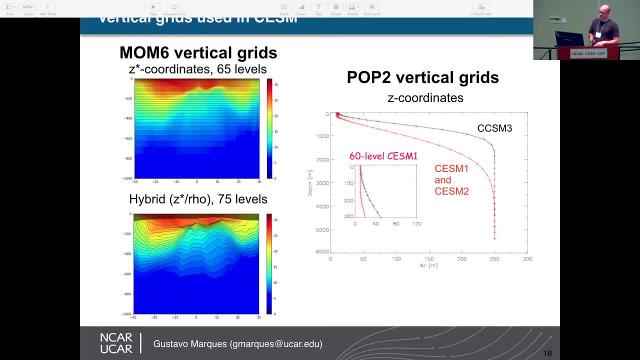 The ones you guys are using are in red- has 60 levels. So that's the grid used, which means you have high resolution near the surface and that kind of decays exponentially with that In terms of surface forcing options for the ocean model. 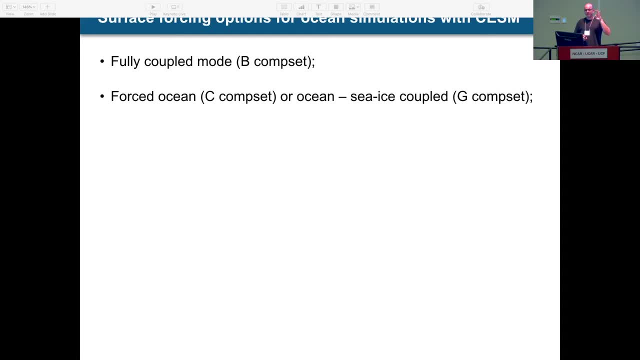 the ocean model. within CSM we have basically three comp sets. You guys are using the B comp set or fully coupled mode, So all the components are active, But in the ocean we also tend to, when developing, specially use all the comp sets. 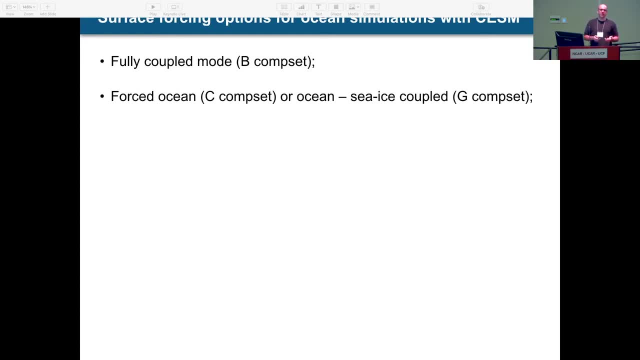 For example, the C comp set has only ocean active. everything else, all the other fluxes, are given by a data component, And the one that we use the most in the ocean, besides, fully coupled, will be the so-called G comp set. 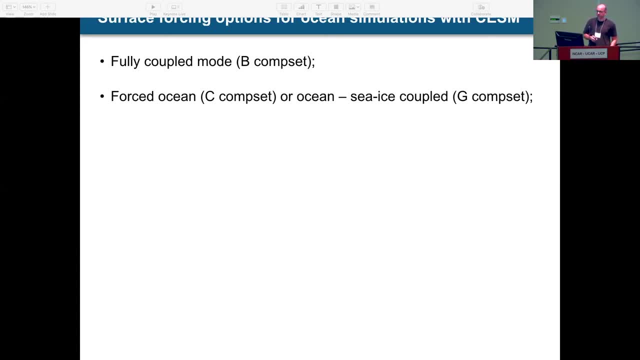 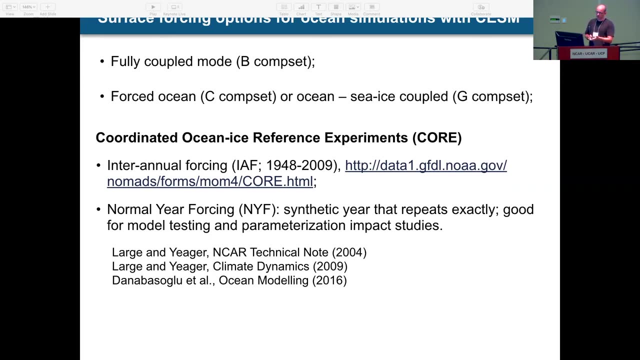 where ocean and sea ice are active. everything else is given by data. And then the forcing protocols. we have basically two different protocols. The first one is the core forcing- like the details here for those of you interesting to look afterwards- And then more recently. 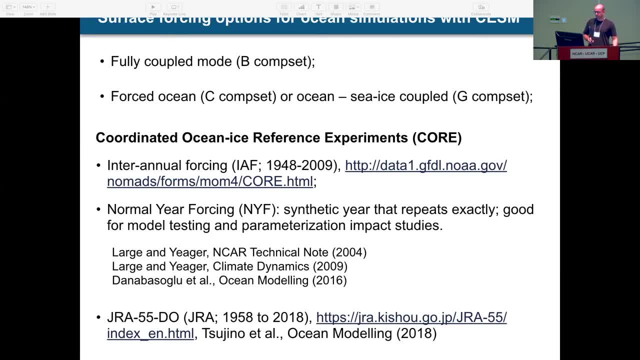 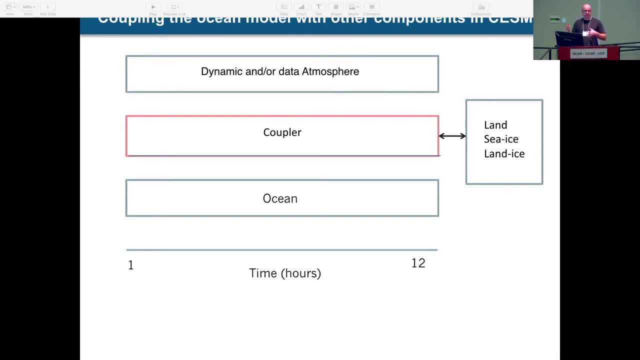 you're using the GRA55 protocol In terms of coupling how the ocean communicates with the other components, So that's a big deal. So how do you, if the ocean is communicating every hour, for example with the coupler, the atmosphere is communicating half an hour. 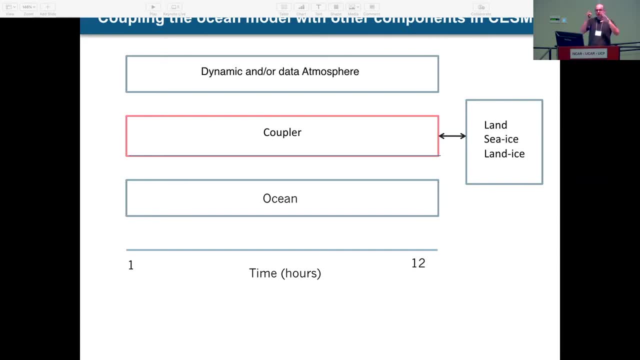 the land model every three hours. how do we make all of things happening And, more importantly, the important properties being conserved? So that's a big deal in CSM and other climate models And the way we do is they can run with different coupling time steps. 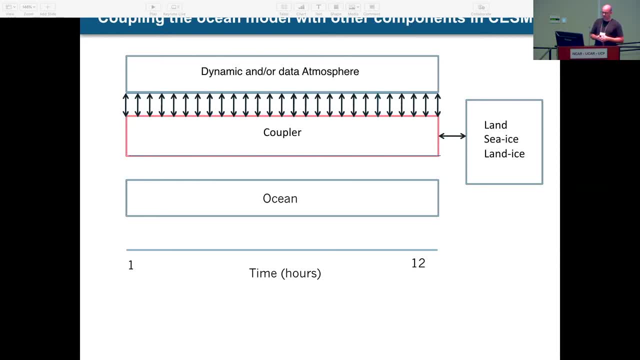 And I think one of the exercise yesterday asked you to change the coupling time step of the atmosphere And the coupler can take care of making sure that things are conserved between when you migrate from one to another, when you pass a flux from the atmosphere to the ocean. 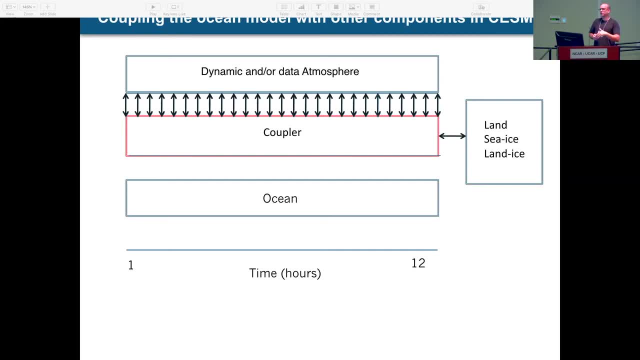 and vice versa. So out of the box, the atmosphere is coupled every half an hour, The ocean is coupled, so every one hour, But again we can change that And the coupler is there to make sure that it doesn't matter the values. 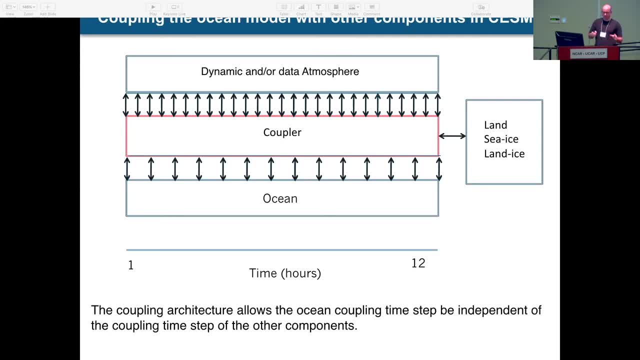 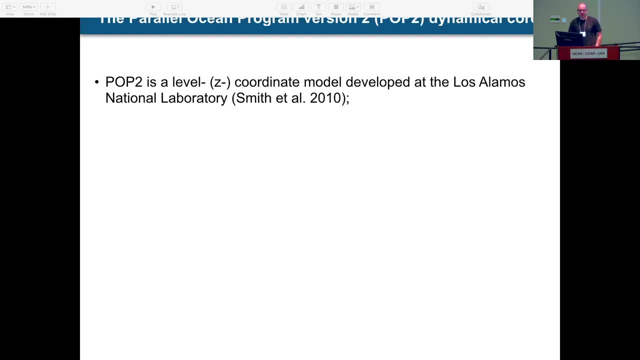 things will be conserved as you go from different values of coupling. I'm putting the ATM and OSHA here, but the same applies for land, sea ice, land ice and et cetera. All right, now moving into the POP model. 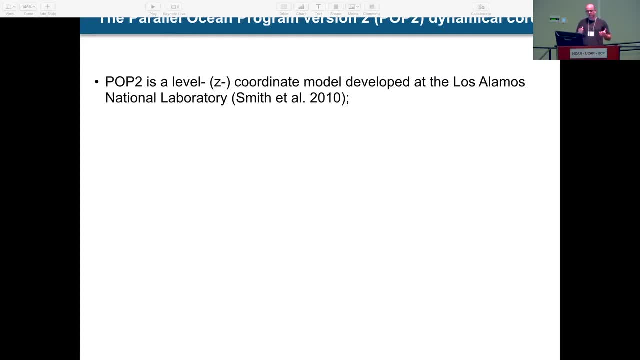 So, as I mentioned, this model is a Z-level or Z-coordinate model. It was initially developed at the Los Alamos National Laboratory. It resolves the three dimensional primitive equations in a general orthogonal coordinate in the horizontal, with the hydrostatic and bussinesque approximations. 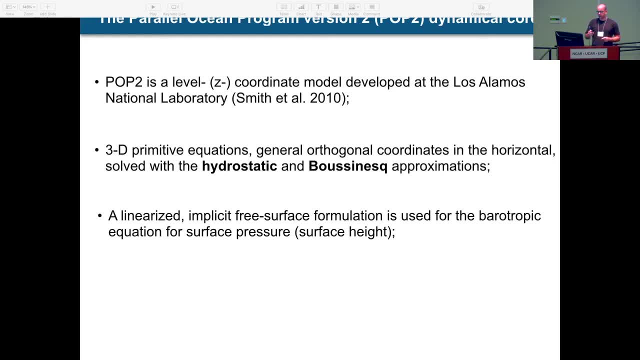 It has a linearized free surface formulation used for the barotropic equation and for the surface pressure. The global integral of the ocean volume remains constant, So that's a consequence Of the bussinesque approximation And also because we have the freshwater fluxes. 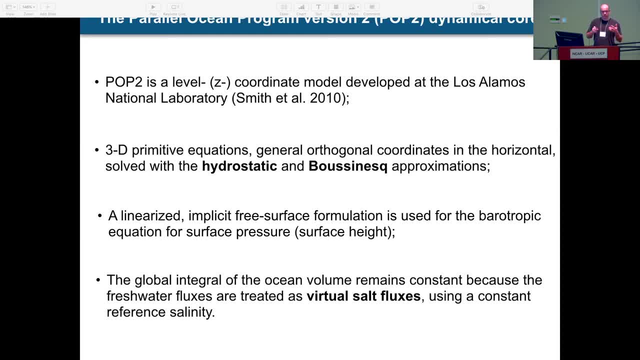 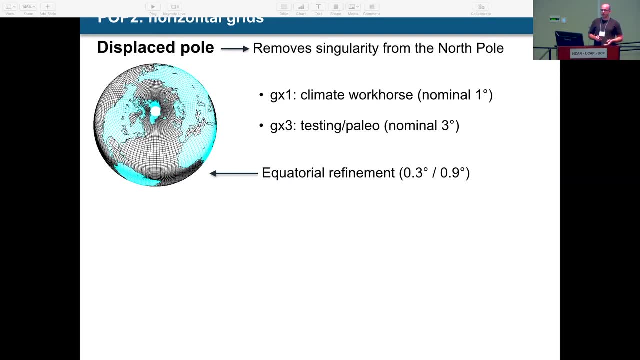 are treated as a virtual salt flux, So using a reference salinity. So now, this is a particular to this model. The new model will not have that approximation anymore or that limitation. These are the grids used in the POP model. The first one is the one you are using. is displaced pole. 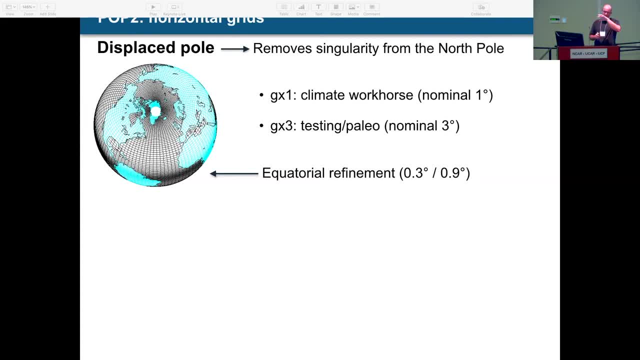 So notice that the pole we started from being in the middle of the Arctic has been displaced to being on top of England or Greenland, And so removes this singularity from happening in the ocean, because otherwise, no, it's a problem. All the cells converge into a single point. 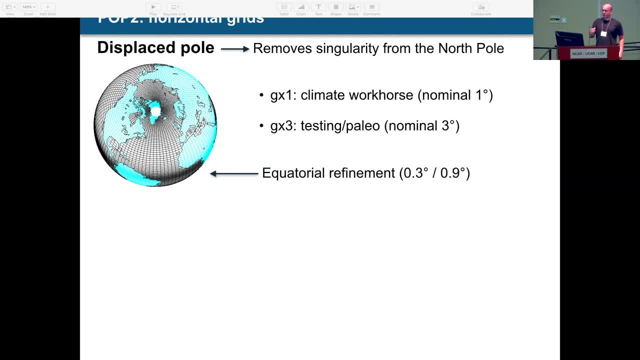 So the GX1 is the workhorse grid that you guys are running. We also have the GX3, which is the three degree version that's used mostly for testing in Pelio, And all of them have a cultural refinement. So near the equator we tend to increase it. 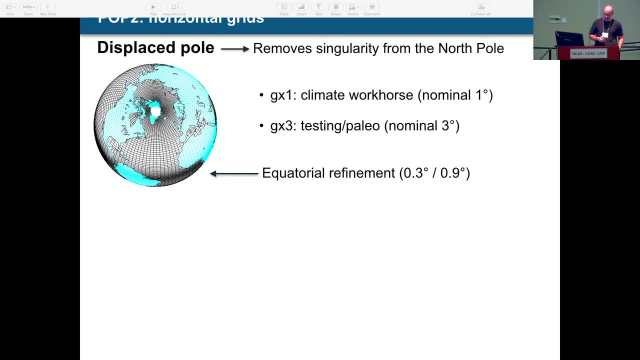 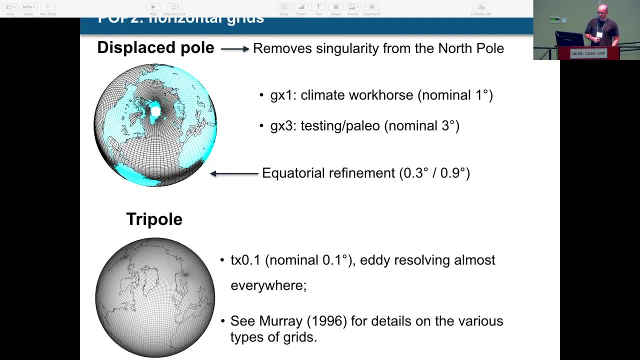 So near the equator, we tend to increase it. So near the equator, we tend to increase it. The resolution to represent the equatorial processes better. The other grid used with POP is the so-called Tripol grid, at one tenth of a degree. 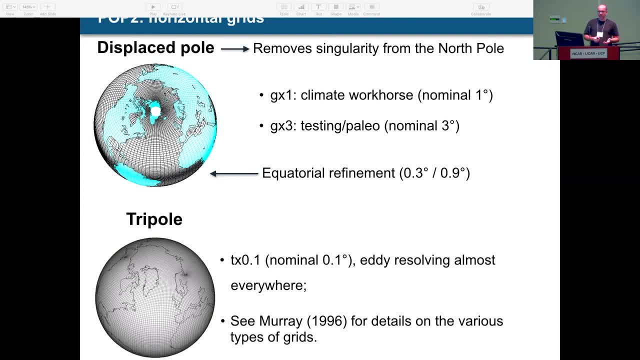 So it's nominal: one tenth Eddie, resolving mostly almost everywhere. If you're interested to learn about the different grids in more details, not just about no, that this was used in CSN, but in general, I'm putting a reference here from this Murai in 1996 paper. 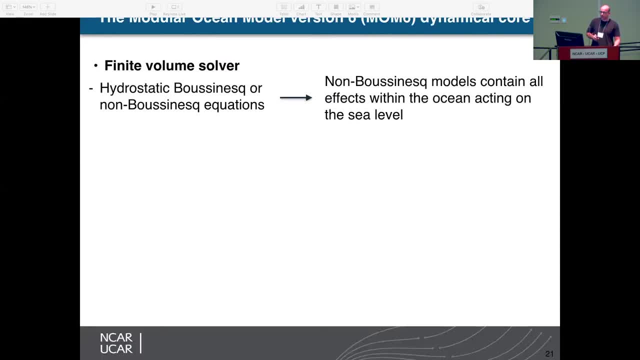 which describes all the types of grids very nicely. Switching now to MoM6, so the new model. so this is a finite volume solver. It has the hydrostatic approximation or the sorry, it has the Boussinesq approximation or the non-Boussinesq, so you can run in both modes. 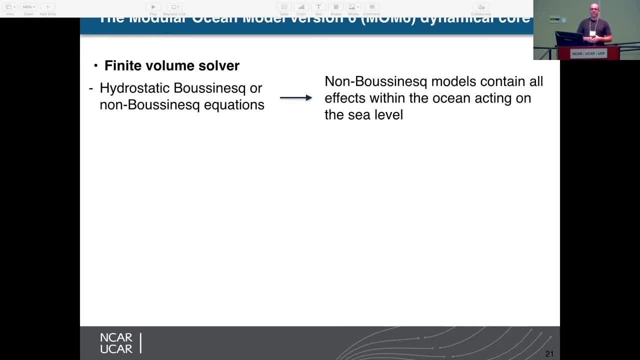 The advantage: out of the box, you run on the Boussinesq mode. If you would like to run on the non-Boussinesq mode, that's mostly for things like studying sea level rise. so the non-Boussinesq let you understand the effect of the ocean. 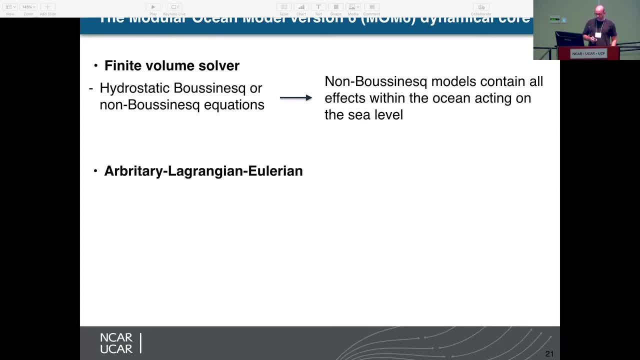 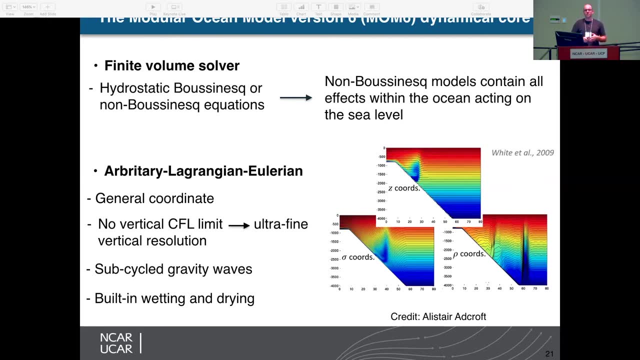 sea level rise in a more complete way, And the main advantage of this model, or the main capability, is the option to use this so-called arbitrarily Lagrangian Eulerian coordinate system. so it's a vertical coordinate system that lets you choose anything you want. 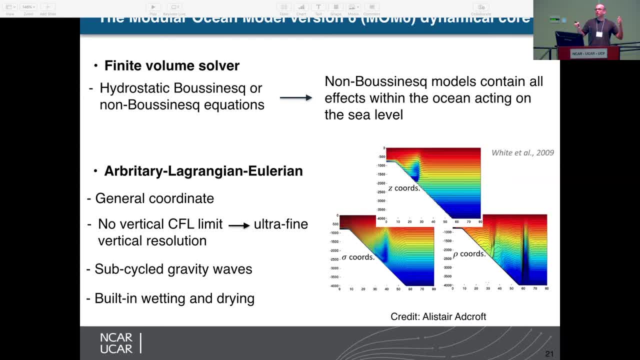 It can be a z, it can be a sigma or it can be a combination of both. The plot on the right shows basically: it's a slope, It's a sloped ocean and you put dense water on the top of the slope and you let the dense 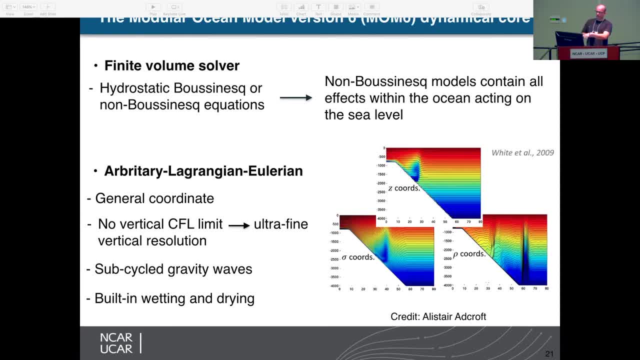 water flow as a gravity current And that is simulated with three different coordinate systems- z-star, sigma and rho- And you can see how that plume flowing downslope differs significantly between the coordinate systems that you choose, just to give you a sense of how that choice, which again is 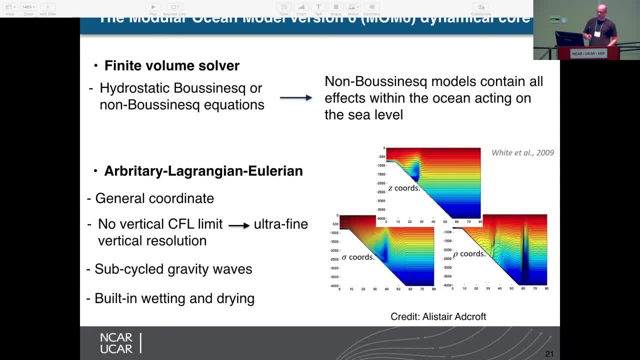 a very important choice in ocean modeling matters for the problem. One of the advantages of this coordinate system is you have no vertical CFL limit because basically, your grid is moving up and down. the thickness of your grid is moving up and down depending on the convergence and divergence of the horizontal flow. 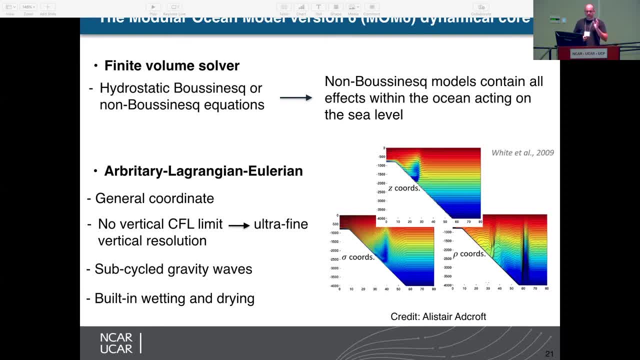 It has the option to sub-cycle gravity waves, And another very nice capability is the built-in wet and drying, which I'll show an example in a second. So things like, for example, a wave. So, for example, a wave. 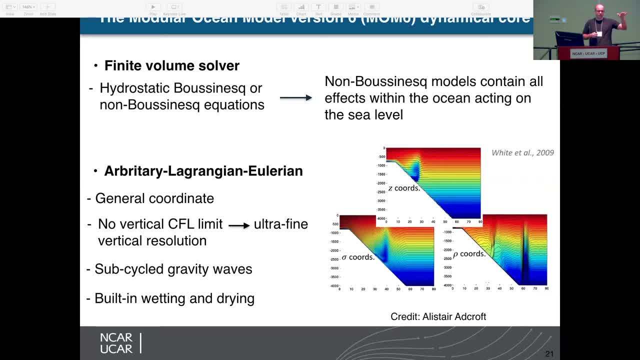 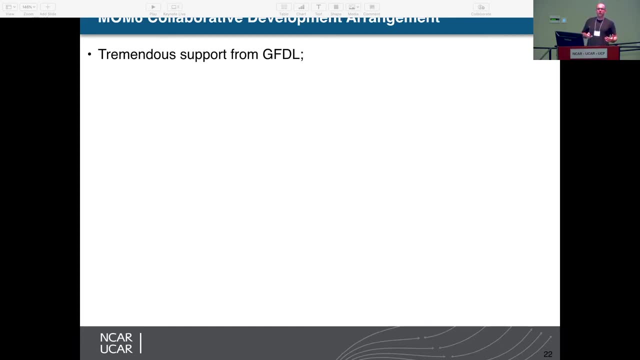 A wave pushing into the shore and then coming back with tides, so making the land points wet or dry. In this model that capability is built in, Unlike the POP model which kind of the development was centralized, you know was focused on. 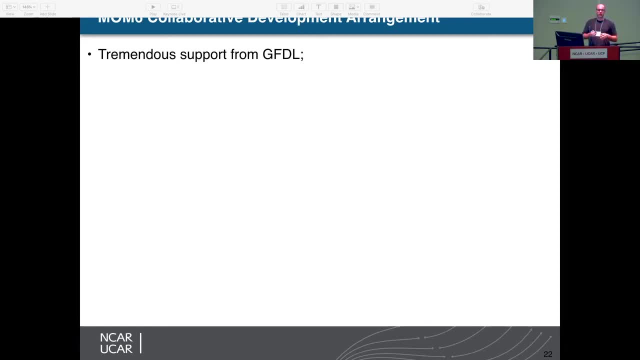 a few places. the MOM6 model is an open development concept, So anyone can develop the model. You can clone the model now and if you see an error or something you'd like to improve, you can create a pull request and then submit your contributions, and it's open to anyone. 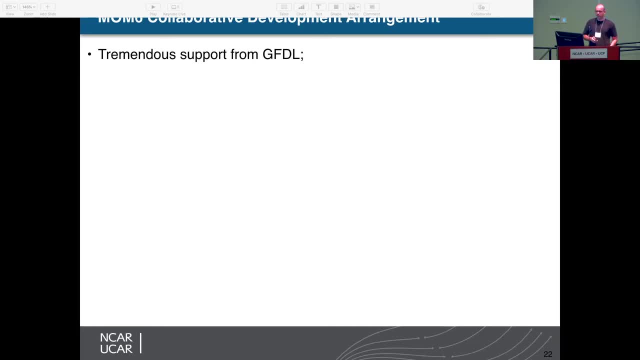 And we have tremendous support from GFGL. we have weekly meetings with them, Not just NCAR. NCAR is not the only center using it. there's centers throughout the US and also overseas using that model and we all communicate with each other. 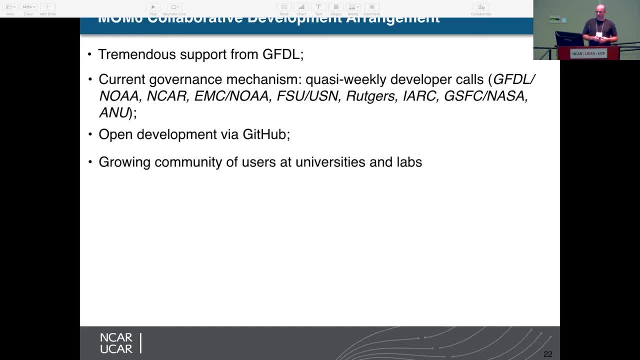 The development is via GitHub. Again, the growing. it's a growing community of users, Universities, labs, and the way we do is there's a central repository called the DAV main repository, and then each center has its own fork of that. 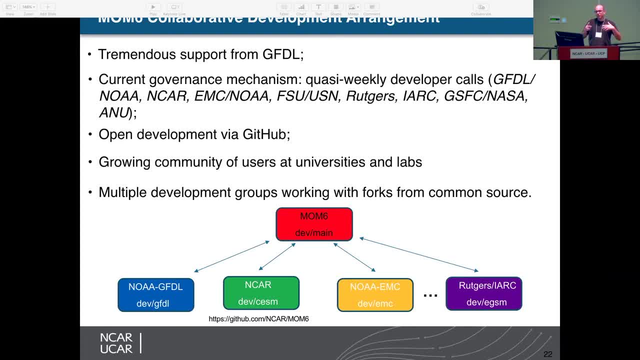 For example, we have one here, NCAR, and then every month or so we all communicate with the main repository and get the features that other people have developed in other places, and vice versa. Now moving to the choices of parametrizations in MOM6.. 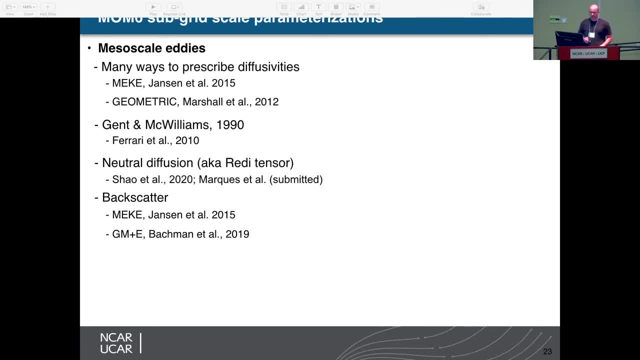 I will not go into detail. I'll let you guys read afterwards and then Peter will cover the parametrizations in more details. But we have a lot of choices for mesoscale eddies, for the surface boundary layer, sub-mesoscale. 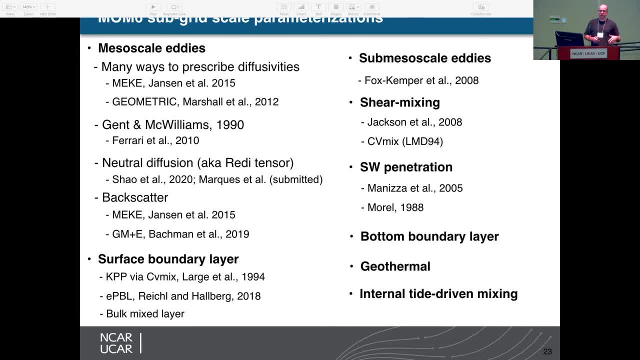 shear mixing, shortwave penetration, bottom boundary layer, geothermal, internal, tide-driven mixing, It's like, compared to POP, the options of parametrizations here are many more and it keeps increasing. Because of this concept of open development, we benefit not just from what we contribute. 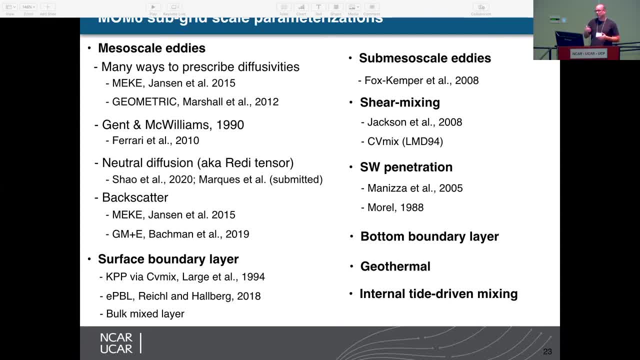 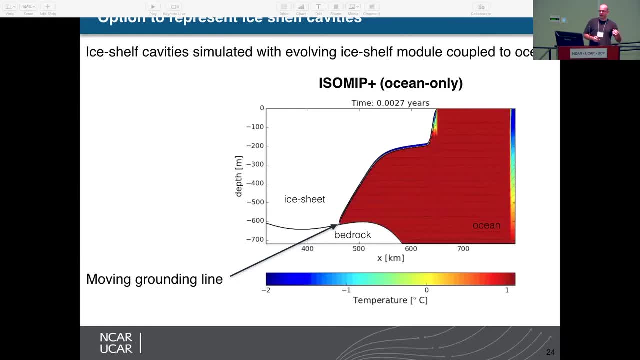 but also from what other centers and researchers contribute. Going back to the idea of building wet and dry, one of the things you can do with that is better represent, for example, the interaction between the ocean and ice shelves. Ice shelves, which are kind of the interface between the land, ice and the ocean. 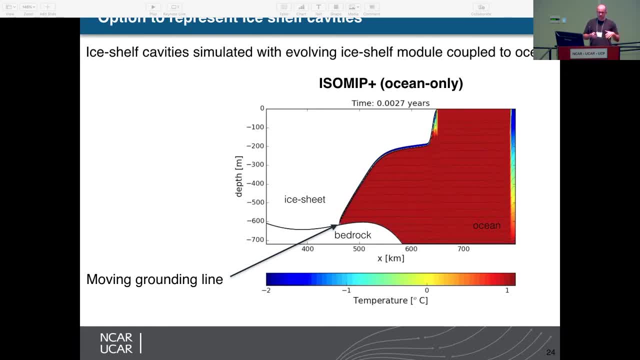 That's what we do. That's what we do. So those platforms of ice floating on top of the ocean, With MOM6, the wet and dry is built in, So therefore you can see there's an ice sheet here on top of the ocean. 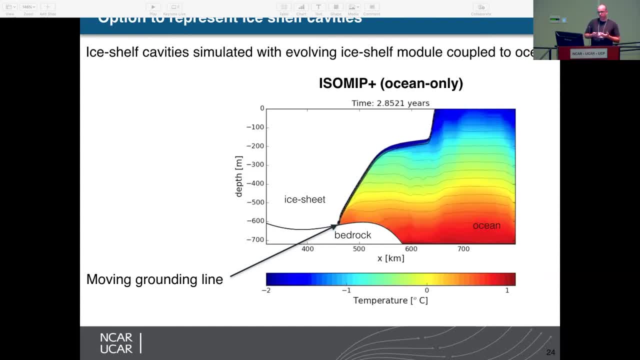 And slowly the ice sheet is melting because the ocean is providing heat And that place that used to be an ice sheet suddenly becomes the ocean. And it is nicely done in this model, which, from other models, is a problem. We don't include ice shelves in the workhorse configuration yet, but that's something. 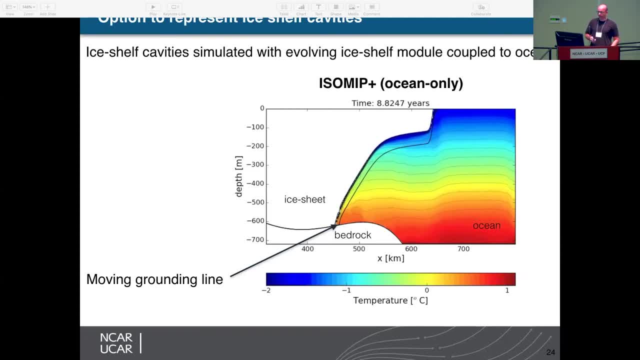 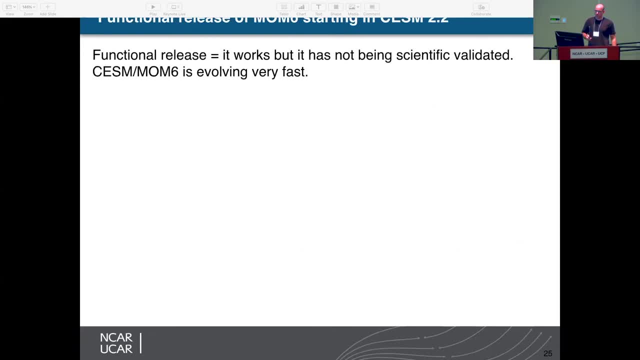 we would like to go into in the future and very important for the climate system when doing the coupling between land, ice and ocean. We have a functional release of MOM6, starting CSM 2.2. And by functional we mean it works, but it has not been scientifically validated. 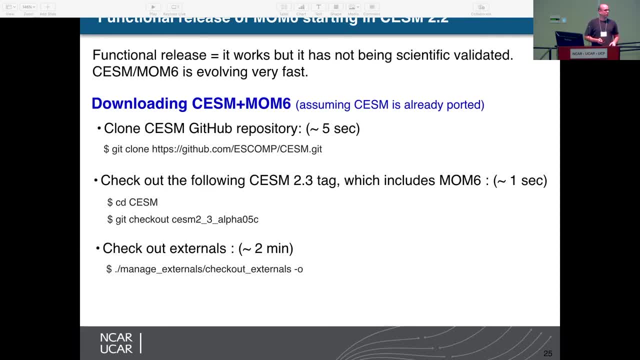 I'm listing here the steps that you need to follow If you would like to start running MOM6 within CSM on Cheyenne. that would be straightforward And that's one of these instructions here. I meant to work on Cheyenne. 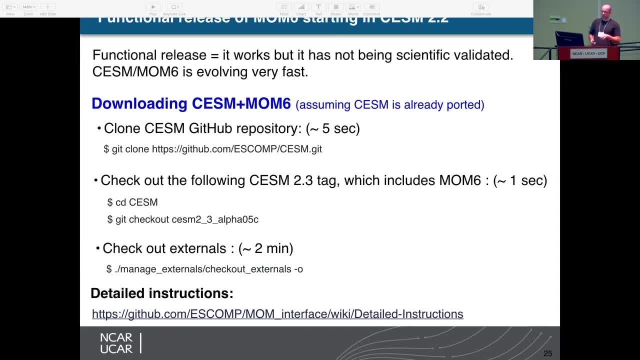 You can go on your own and try to reproduce what's in here, And I also put a link here to a full, detailed description of how to do that. Again, do that on your own. If you have any questions, please feel free to reach out to me. 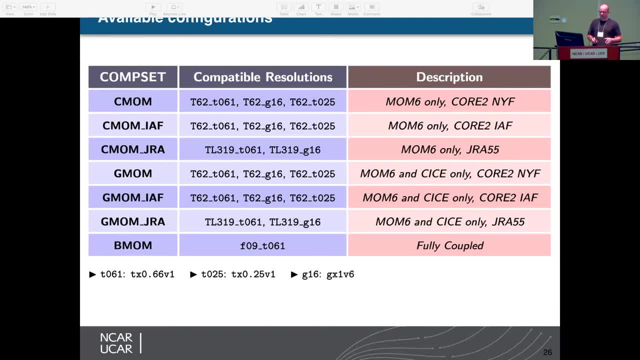 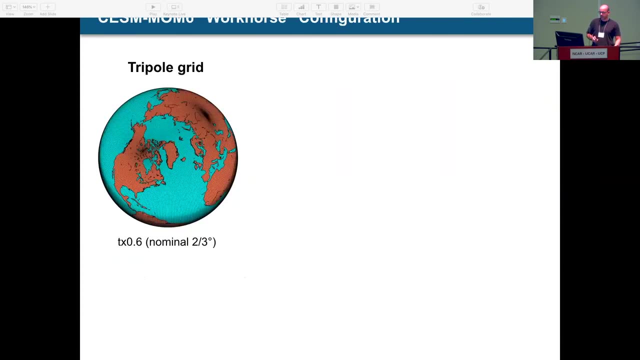 Briefly, those are the concepts that we support with MOM6.. You should be familiar now with the concept of CompSat. You can read on your own what each of those mean And again, if you have any questions, feel free to reach out afterwards. 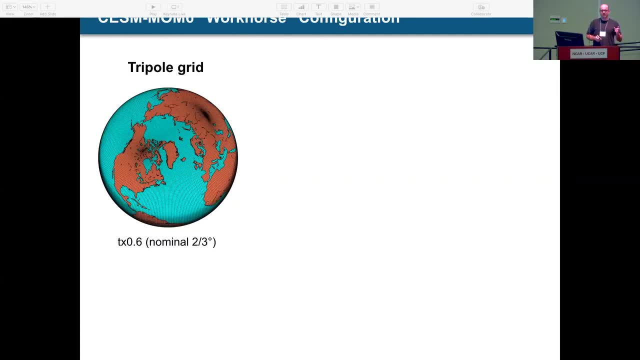 The grids used with MOM6, so we have basically two or three grids that have been developed. now. The first one is what's used in the workhorse of simulations with MOM6, is the GXO6, it's a tripolar grid. 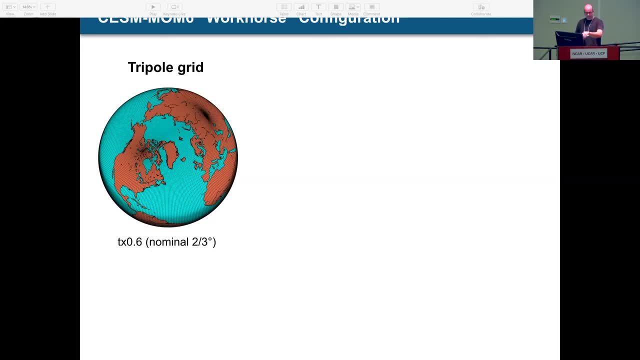 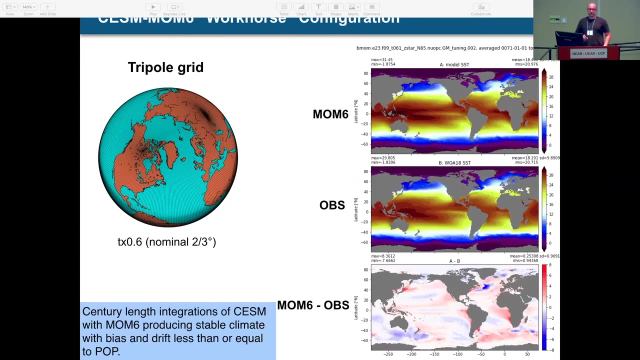 It has three poles, so one on top of Russia, the other one on top of- I think that's Canada, and then we have the one on the South Pole, So that's why it's called a tripolar grid And that's the workhorse configuration now has a resolution of two-thirds of a degree. 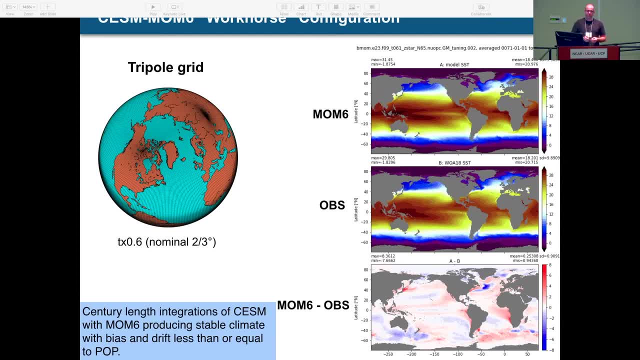 in the horizontal again, with equatorial refinement up to one-quarter degree. We have already performed century-long integrations with CSMM6 in fully coupled mode And I'm showing you here a plot on the right of the SST bias compared to the observations. 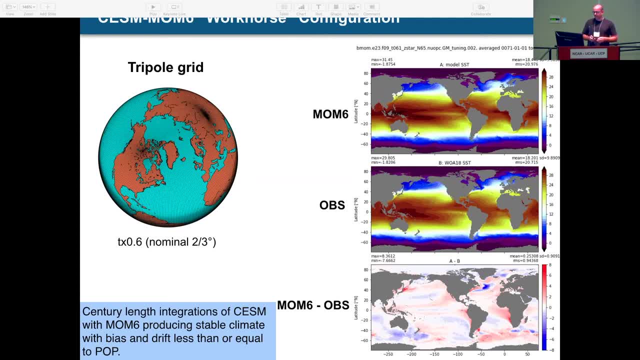 over the last 30 years of the simulation And the bottom line is, as of now, it's producing a climate with bias and drifts very similar to what we get with POP. We are very actively working on this configuration with other components towards CSM3. 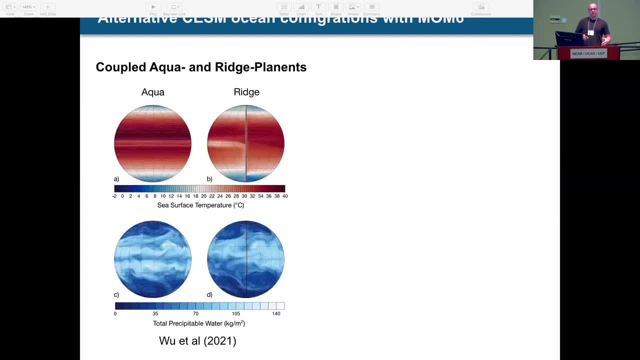 In addition to the global workhorse configurations and the high resolution, we also have these alternative configurations with MOM6.. The first one is the so-called coupled aqua rigid planets. So the left plot shows the aqua planet. So basically you have two caps on the poles and everything else is water. 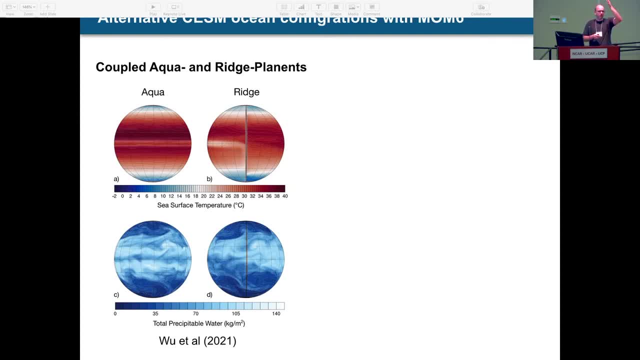 And the right plot shows the rigid case. so then you have only like a ridge that goes from north to south, And those are fully coupled couple simulations and you know it. and this was a contribution from a grad student, xiaoning wu, that was an asp visitor, and she, she did that during her phd and, for those of you interested, 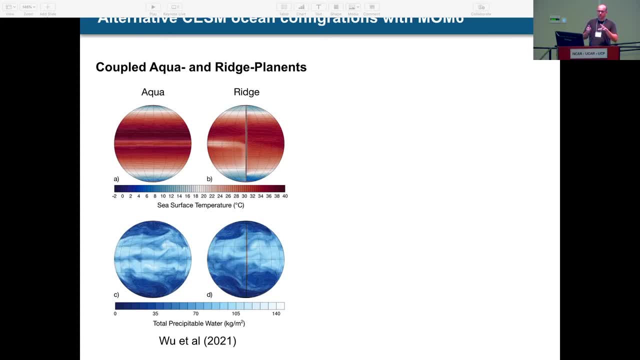 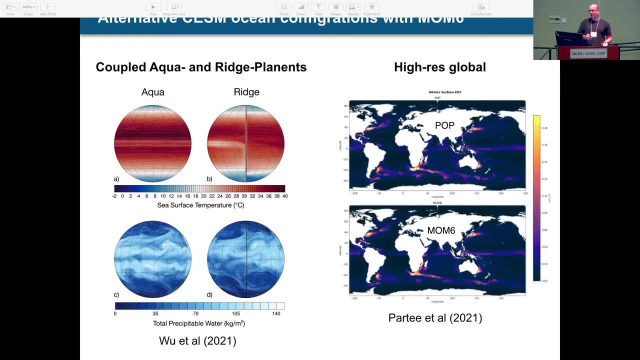 we, we can, we can talk more. we are currently working to develop a more user-friendly way to come up with these idealized planet configurations, or quasi aqua planet configurations. i already mentioned we have high high resolution configuration with mom six. two- and this is just to show- is the same grid. basically, we're using pop and mom, so the top panel shows that this is. 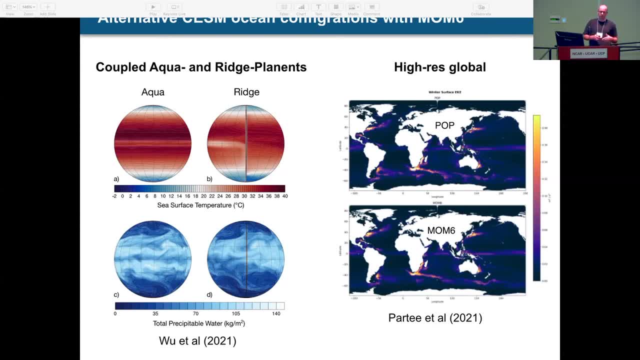 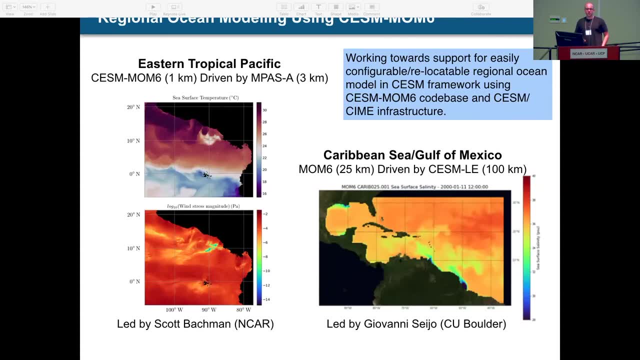 eddy, kinetic energy in the pop model and on the bottom, same grid for the mom model, and you can see they are very similar. we also have the option to simulate, to perform regional simulations with, with mom six, so all of these are the same dynamical core. 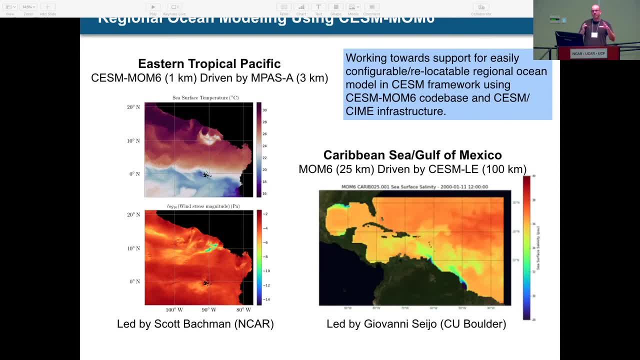 you can do all of these types of simulations within the same csms and box. we have two working configurations, regional configurations at the moment: the east tropical pacific, one that's led by scott bachman from ncar, and the caribbean sea gulf of mexico. 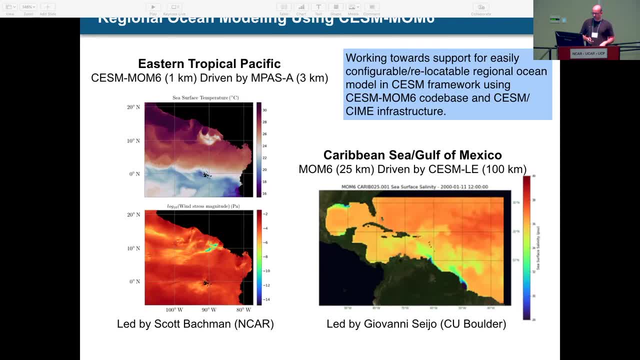 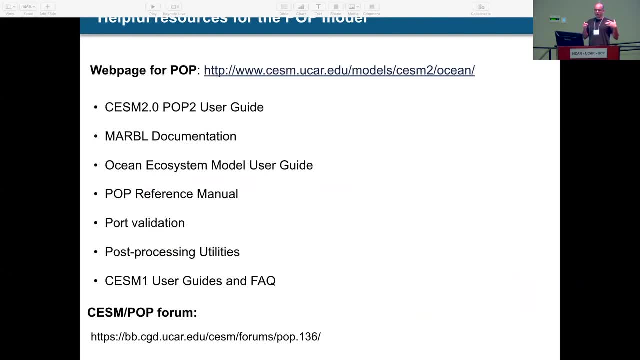 configuration which is led by grazia from cu giovanni seo. in terms of resources, these are all the resources available. if you're interesting working with the support model, so go to thexygov, to the webpage. you have user guide. I didn't mention about the marble configuration. 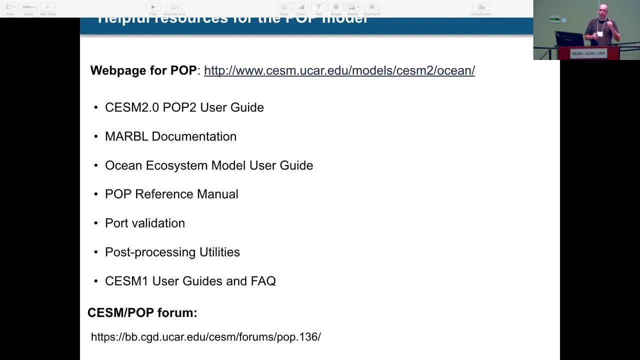 or the biogeochemistry. You will learn more about that tomorrow with Keith Lindsay, But no, the biogeochemistry model is coupled to the OSHA model in a way. it's, of course, has been implemented for POP and we are currently implemented for MOM. 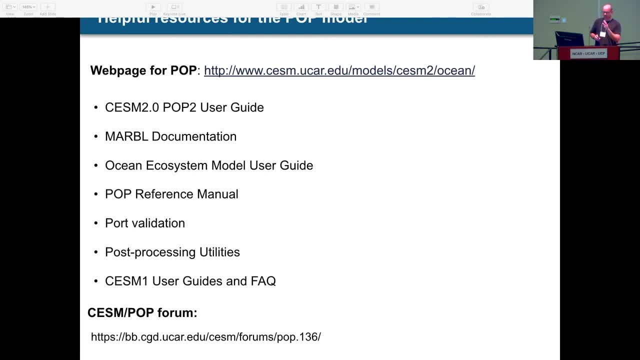 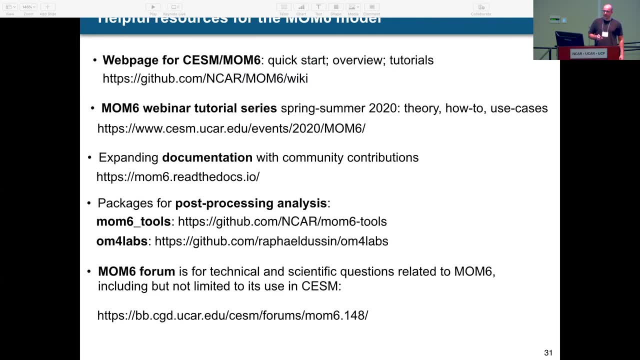 Here's the documentation for the marble documentation- and Keith will talk more about that- And there's a forum if you have questions on the POP model that I put the link at the bottom here and the same type of resources for the MOM6.. There's a Wiki- how to get started. 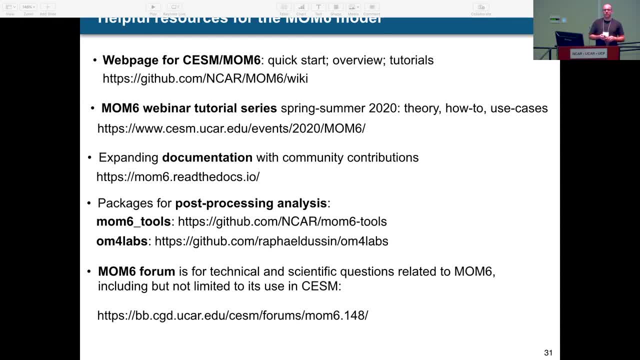 some overview tutorials. We also performed a series of webinars in 2020 with a lot of talks, and those are made available on this URL as well. The documentation keeps expanding. There's packages for doing post-processing analysis And also if you have questions. 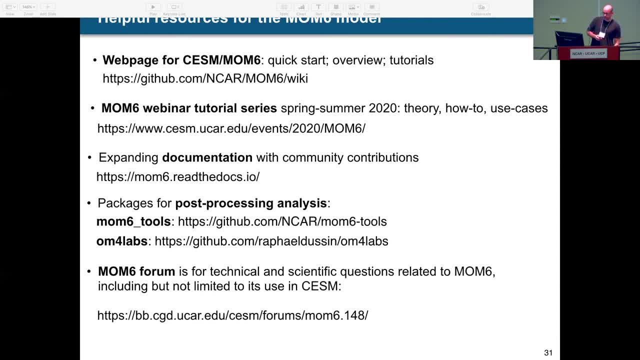 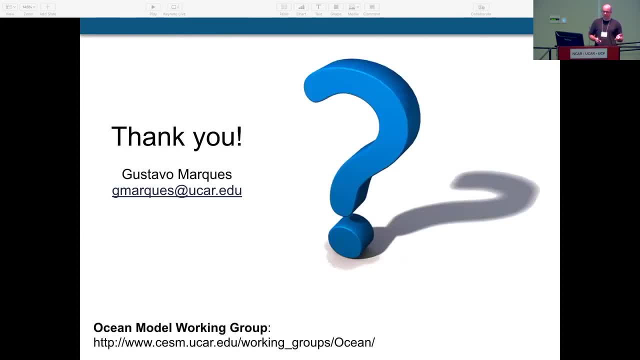 there's a forum within the CSM on the OSHA model working group website. These are the references And I'm happy to take any questions. Thank you for listening. Once you engage with the OSHA model working group, here's the link. 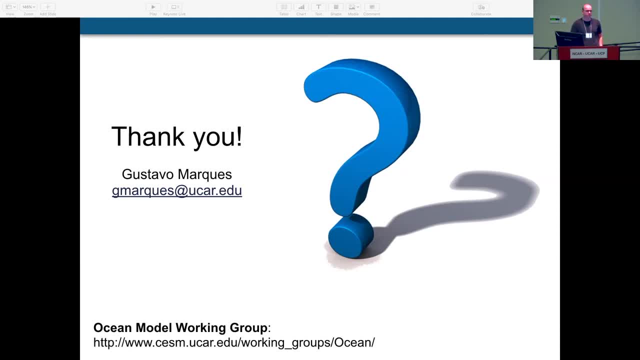 Feel free to go and subscribe and you will be receiving the emails from us. Great, thank you so much, Gustavo. If people have questions, please come to the mics. Obviously a pretty complex thing to understand how the OSHA models. 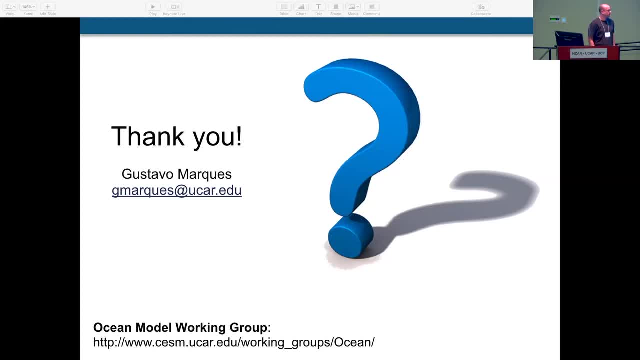 being run and now movement from POP to MOM is like a big component of what we're doing as the efforts within NCAR. So, yep, Yeah, I was curious, like I'm mainly using the MS3 models, and it seems that like, as you mentioned, 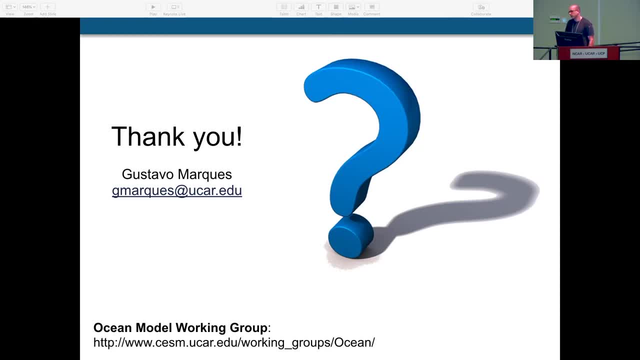 in the weather scale for the ocean it's like less than one degree, but with the MS3 model it's mainly one degree And I was wondering, like in the copular, does that control these different resolutions? and like: is there this like? 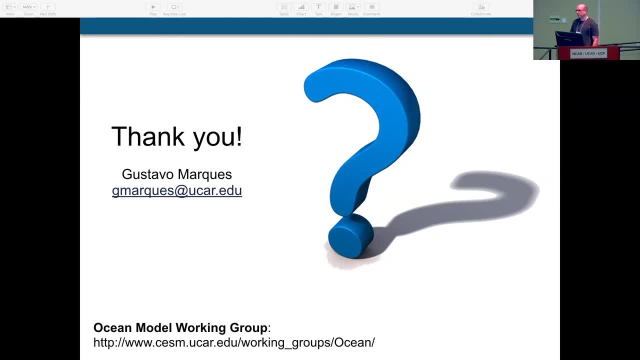 is there this like this kind of, you know, like interaction between the weather scales, or how does it work? Yeah, so the way the coupler works up to now, like he always uses the highest of the two resolutions to interpolate- 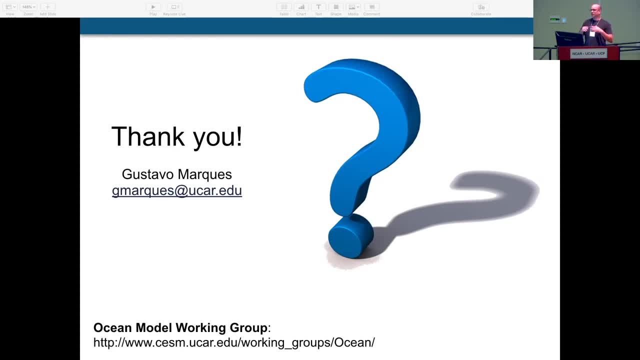 from one to the other and then propagate that. So if the ocean is receiving flux from the atmosphere, the coupler will interpolate that flux into the ocean grid and then propagate. Now, very recently, we have a capability of combining the two grades. 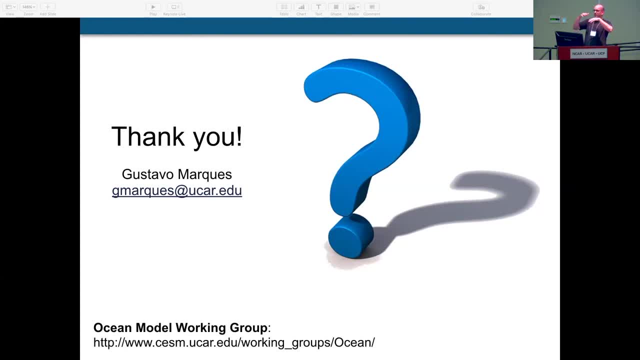 So it's: we basically overlap. the coupler grid is a combination of the atmosphere grid and the ocean grid, And then we'll basically superimpose those on top of each other. So it's a much higher resolution than both the ocean and the atmosphere. 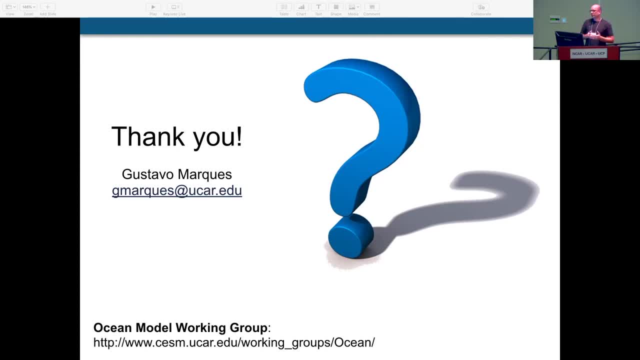 And that will improve the fluxes. I don't know what is the limitation of like. not including this, like you, might, for example, lead to not representing the winds very well near the land ocean boundary, for example, because of the different resolution. 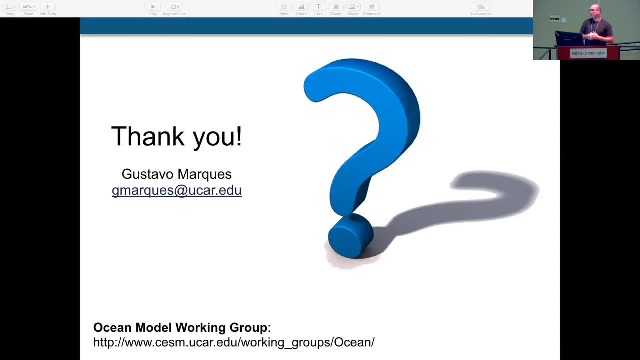 But with this new capability this type of problem will go away. Does that answer your question? Yeah, yeah, Thank you. So in the atmosphere model we learned the other day that they have these regional grids like the continental United States grid. 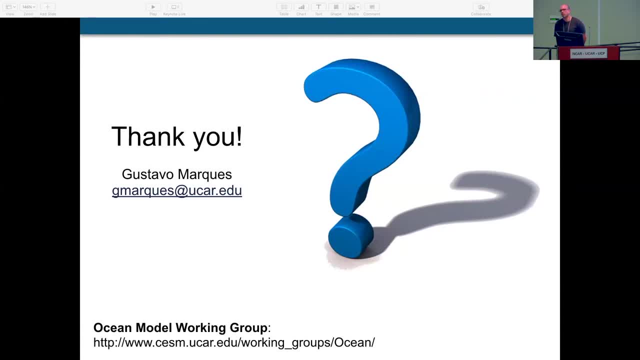 where they have high resolution over one area and very coarse resolution over other areas. I was wondering if something similar is possible within MOM, although I think you mentioned that grids are challenging in ocean models. Yeah, So for both MOM and POP we use the curvilinear grid. 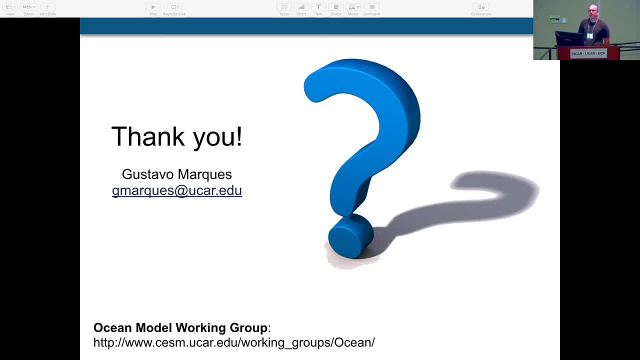 It is a structured grid, It's not an unstructured grid. An unstructured grid is what allows one to do this type of refinement of going like one kilometer in one region and 10 kilometers somewhere else. So a curvilinear grid or a structured grid. 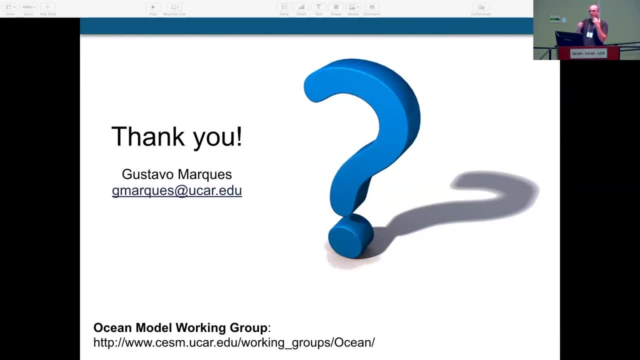 gives you some leverage on changing the resolution a little bit, however, not to the point where you can do things like what they do with the unstructured grid. So the answer is no. we cannot do the same in the ocean model with the type of grids that we support right now. 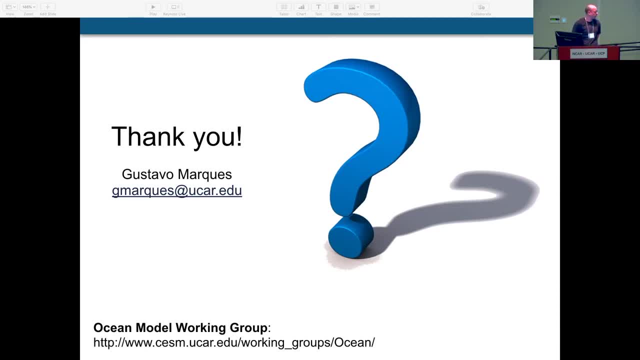 Thank you. Sorry, Gustavo. is there anything to do with ROMs and MOM coupling, Because I know having the nested gridability within POP was something that we were developing and going forward. Is there an effort for going from MOM to ROMs? 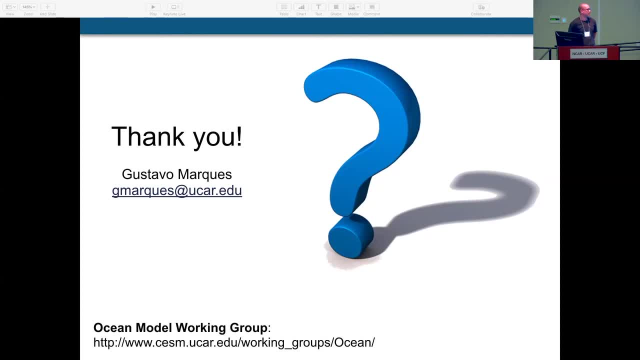 So actually MOM is now being used by the coastal community as a regional ocean model. There's over 20 people- researchers, NOAA and universities- working on that And there's a weekly meeting. There's a biweekly meeting devoted just for regional MOM6 capability. 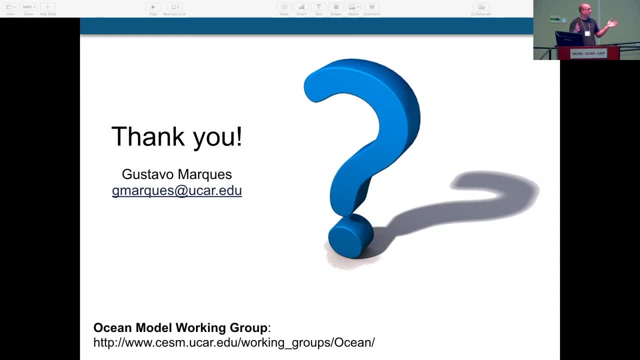 So it's basically doing what ROMs is doing. It's not as wide as spread at the moment, but it's growing very rapidly. So soon you will be able- just within MOM6, to go from global to regional. And is it going to be nested or coupled like two-way coupled? 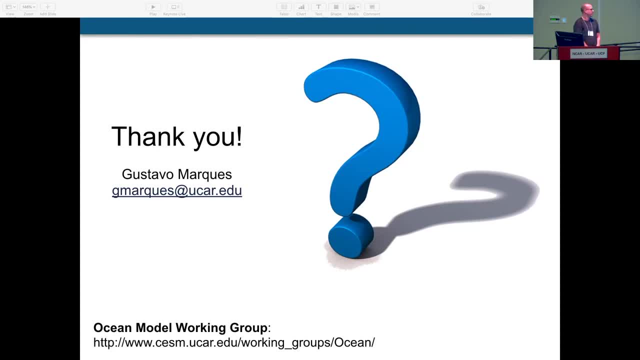 We would like to do that. We don't have the. as far as I know, that has not been put forth yet. Yeah, that would be awesome. It's a very challenging problem to do the two-way nested. Great Thanks. 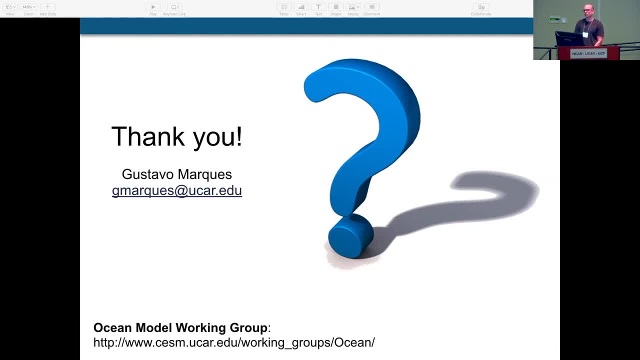 That capacity for freshening or wetting of? I am assuming that was around Antarctica, that simulation you showed. does that improve historical sea surface temperature? Do you have any predictions or what effect has that had? Yeah, so that was an idealized simulation that I showed. 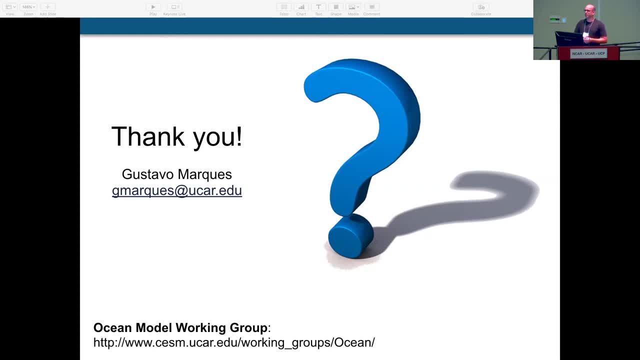 which it was representing processes that happened around Antarctica. as you pointed out, However, none of the climate models have this capability enabled yet, So I cannot answer your question because we don't. we haven't done that yet. Do you have a hunch as to if it would improve the nation? 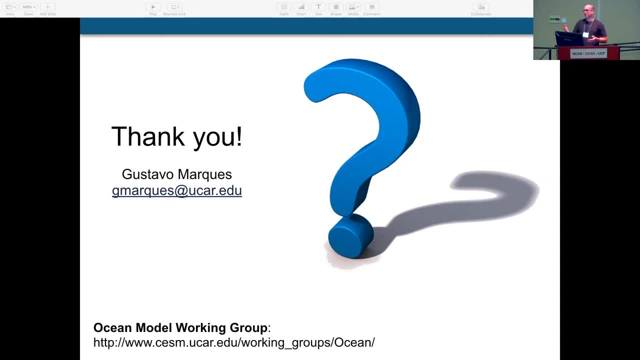 No, I think you. I think it would play a huge role in the formation of Antarctica bottom water and sea ice around Antarctica and therefore things like overturning circulation For surface temperature. I'm not sure, Maybe around Antarctica, but not much, far from there. 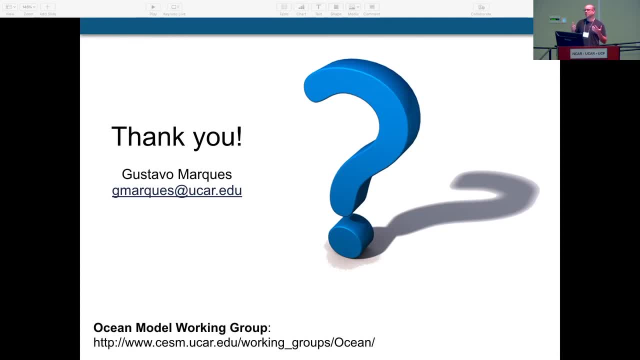 I don't see how that would affect Surface. temperature is just so given by the flux that you receive from the atmosphere. So it's like a couple, A couple problem between the ocean and atmosphere, mostly The ice shelf. I don't think it would impact that. 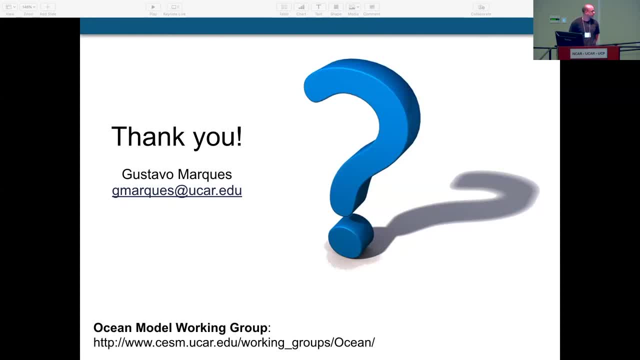 That's my guess, But would it be beneficial for the ice shelves, Like being able to model the ice shelf retreat or extension For the ice sheets? yeah, Yeah, it would definitely be Like things like sea level rise, like this capability.